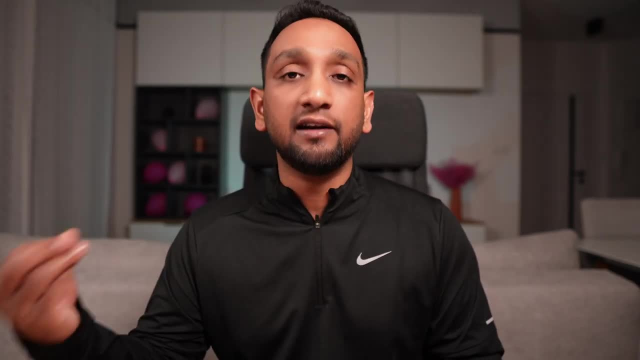 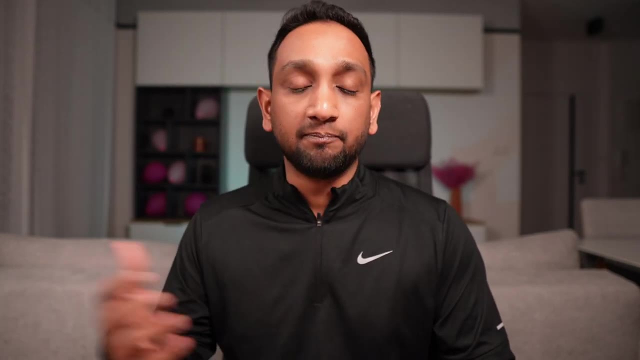 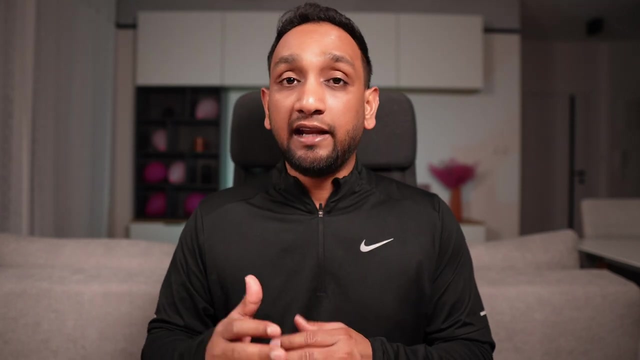 that database. then we could have avoided this kind of data redundancy. okay, So I hope this is clear. Now let us understand designing a database. What does that exactly mean? right So database? mainly, the main purpose of having a database is to store data. right Now, database. 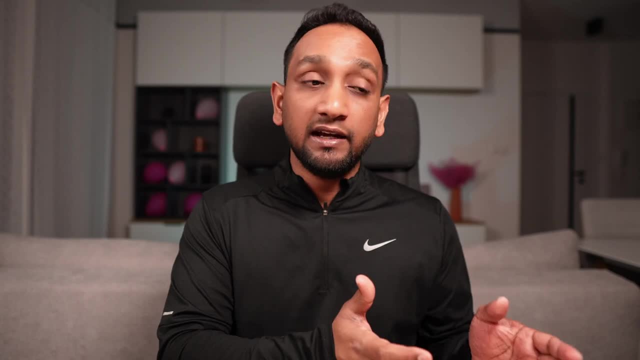 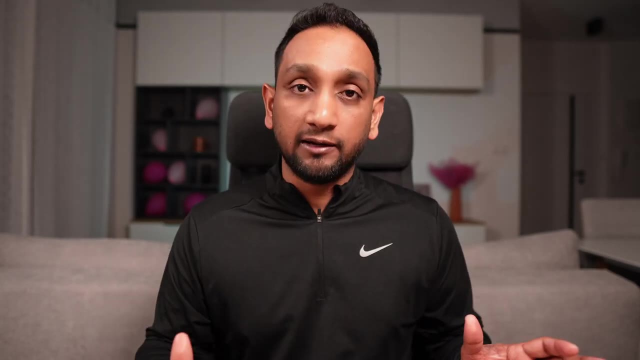 will store data in tables, So there are databases. databases will have tables and table is the object which is going to store your data right Now. it does not mean that you just create one single table to store all your data right. Generally, what we do is based on our requirement. 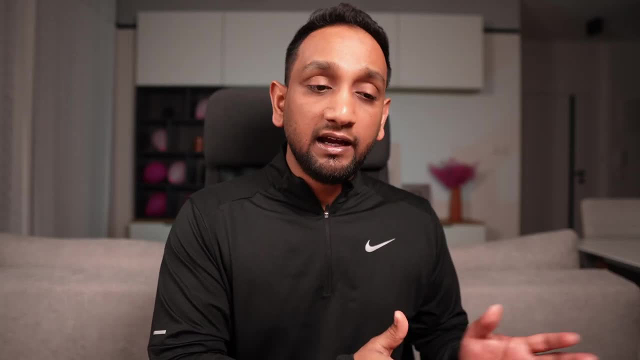 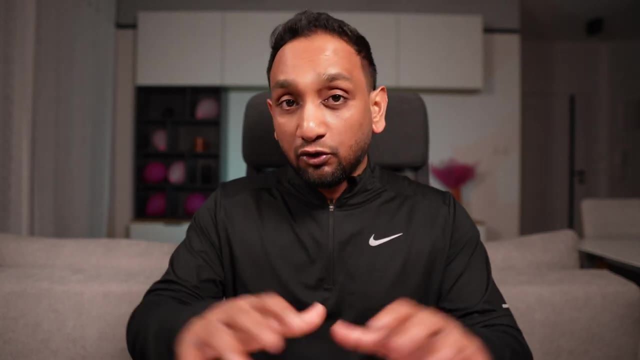 or our project need. we would be creating a list of tables and we would create each table to store one type of data And then we would try to build relationship between these tables. right Now, this whole process of coming up with multiple tables to store a specific type of data and then 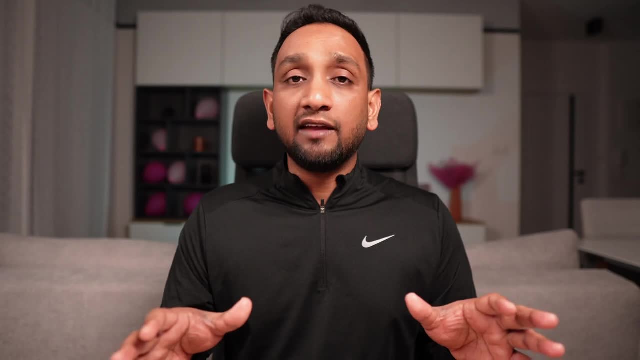 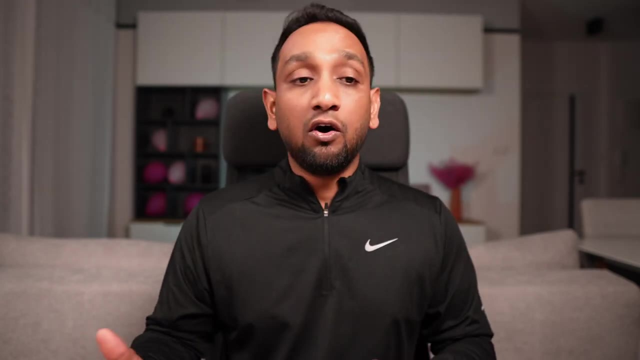 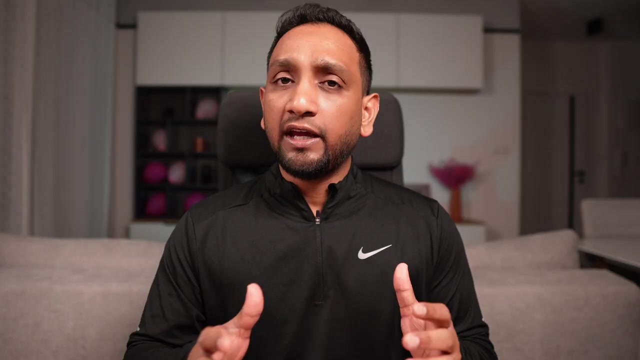 building relationship between these tables can be called as the process of designing a database. right Now, if I have to summarize, I can say that normalization is the process of effectively designing a database such that we can avoid data redundancy. Okay, so now you understand what. 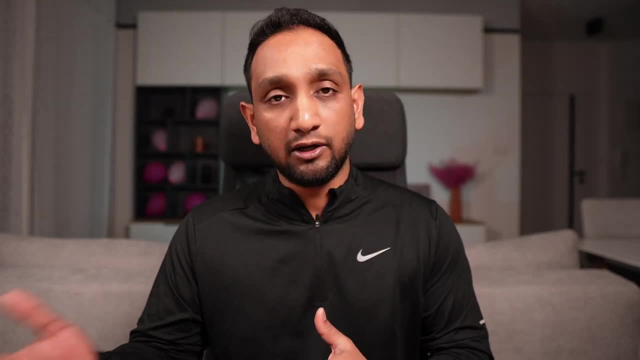 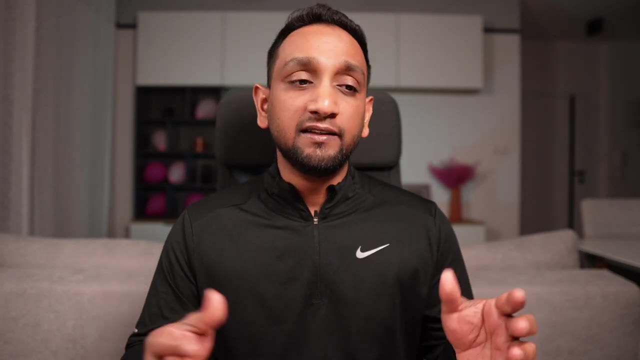 normalization is. let us understand the different levels of normalization now. So let us say you have a denormalized data set and you have been asked to normalize it Now. there is no magic click and your database automatically gets normalized. Generally, what you need to do is 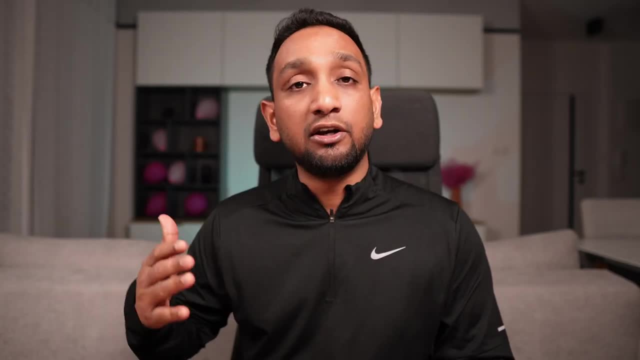 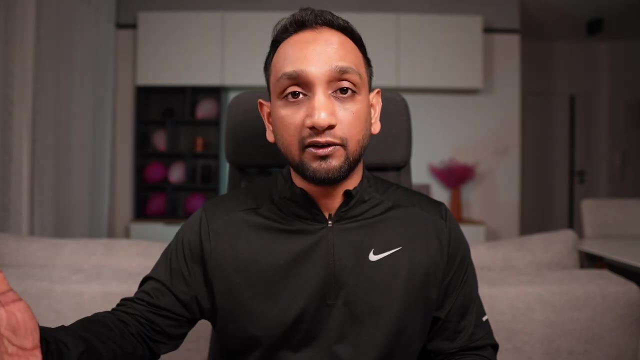 you need to follow certain rules. there is a step by step rule that you need to follow in order to normalize your database. Now, generally, what happens is there are different levels of normalization that you can do on a database. Okay, now, each of this level, we will have certain rules. As soon as the database will satisfy this rule, you can say that the database is satisfying that particular level of normalization. Now generally we have: the first level of normalization is called as first normal form, then the second level is called as normalization. 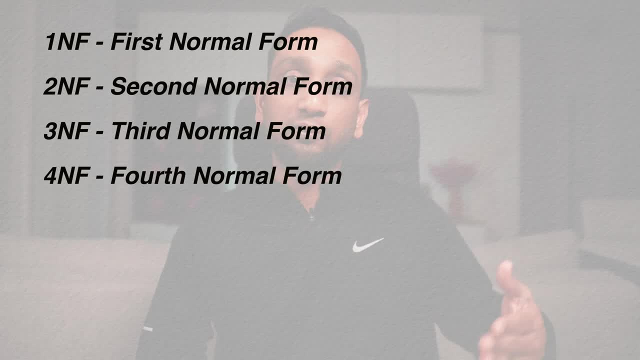 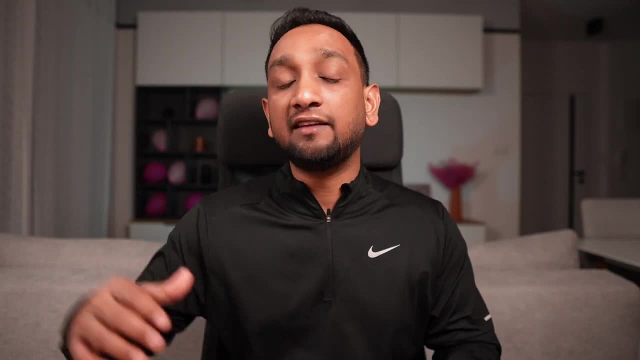 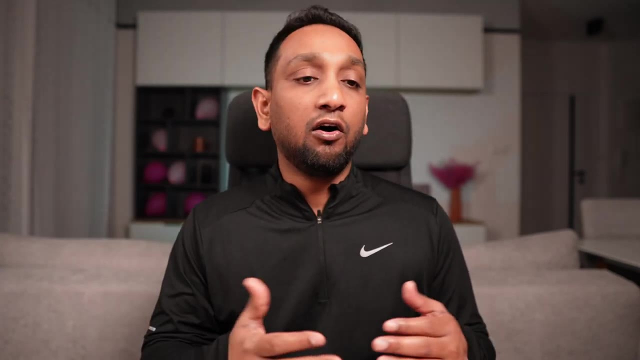 Then we have third normal form, fourth normal form- BCNF. fifth normal form, sixth normal form, etc. Right Now, each of this normal form basically is a level of normalization. Under each of this level, there are certain rules that we need to follow. as soon as, so, let us say all the rules. 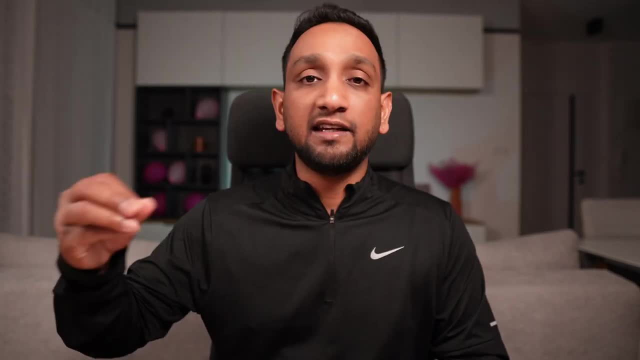 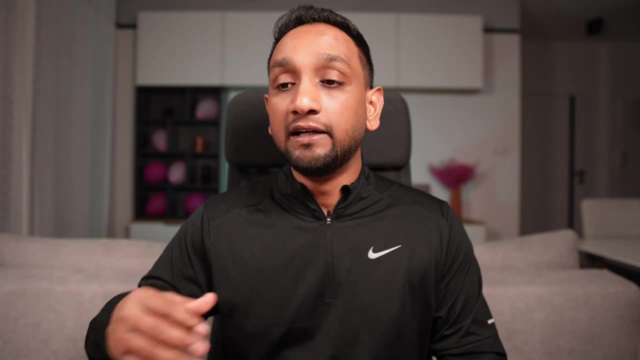 of the first normal form. if a database satisfies, then we can say that that database is in first normal form. As soon as that database will satisfy all the rules of level two, that is, second normal form, then we can call that database in first normal form. Now let us say that the database 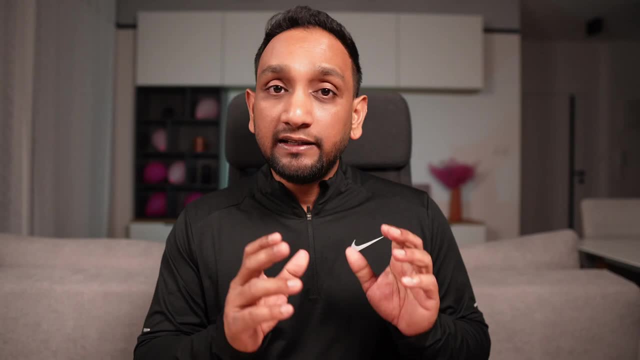 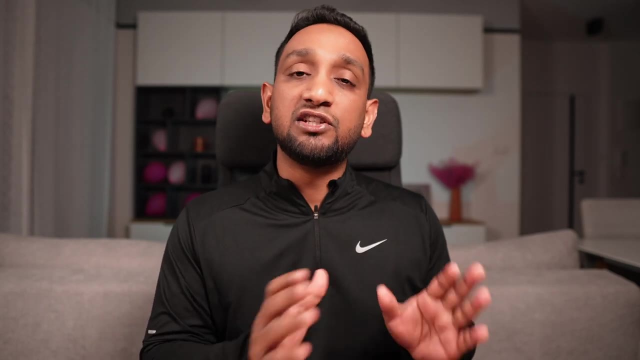 to be in second normal form. Okay, Now, one thing that you need to remember here is, even though we have so many different levels of normalization, the golden standard of normalization is generally third normal form. Most of the companies today try to normalize their database only until third. 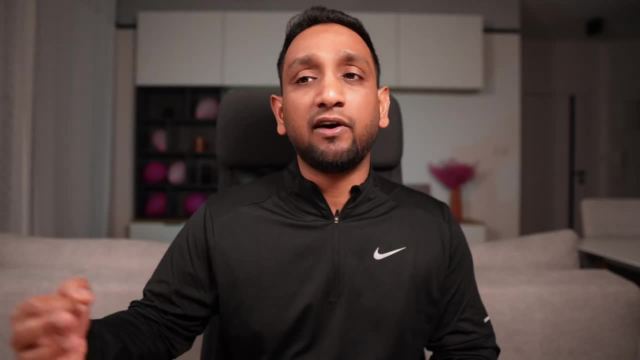 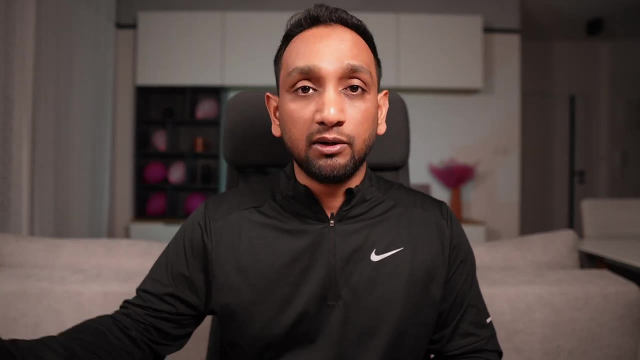 normal form. there can be some specific cases or specific requirement where a company or an organization or a project team might want to normalize your database even further than third normal form, But in general, in most cases, generally the normal form is going to be in. 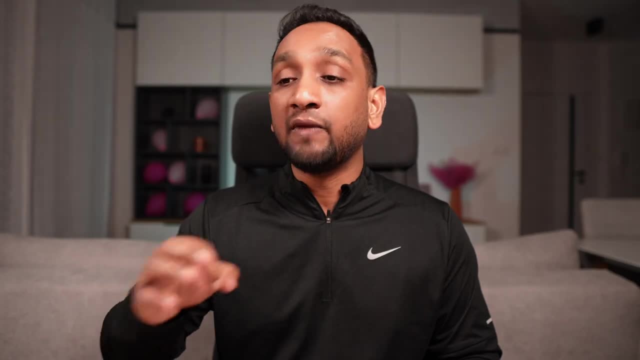 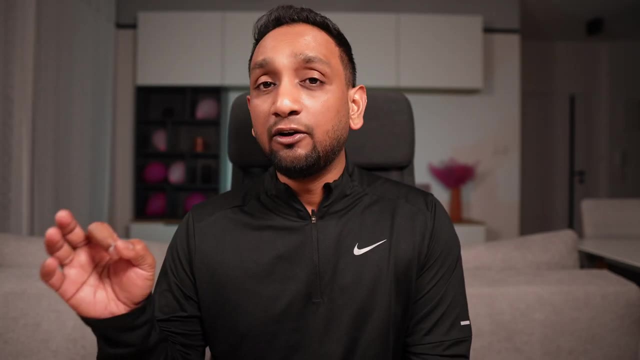 third normal form, And that is why, in this video, I'll be talking only until third normal form. Okay, so now, having said that, I hope you understand all the basics. Now let's look at a proper example of denormalized data set that I've taken from Kaggle, and we'll try. 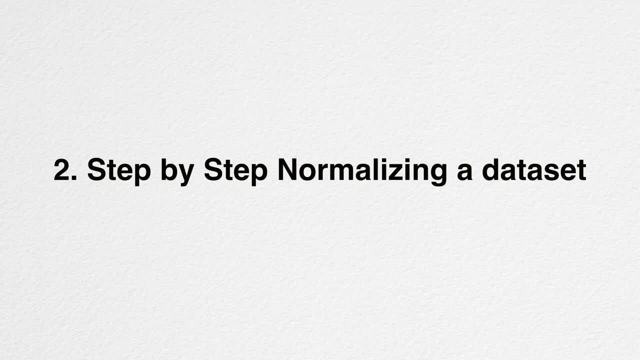 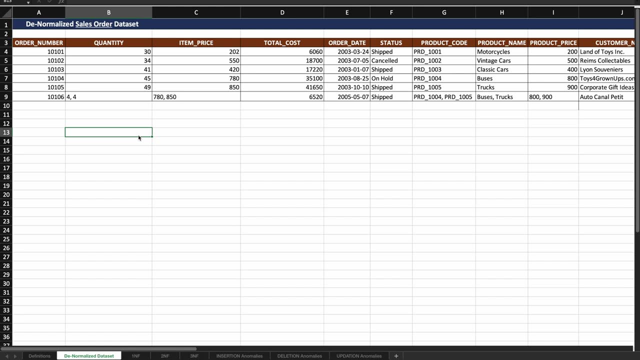 to normalize it using different levels of normalization. Okay, so, as you can see, this is the denormalized data set that I have taken from Kaggle. Now, of course, when I took from Kaggle, it had a lot more records, I think 1000s of records. 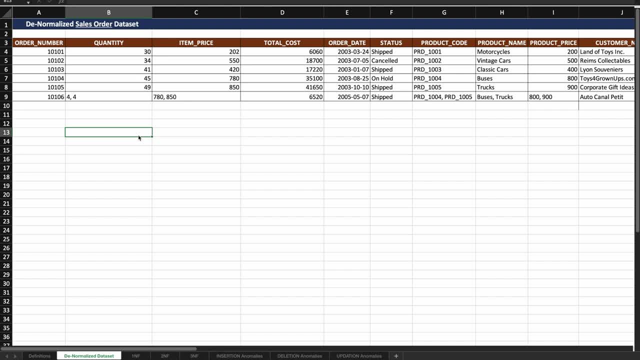 but I have just taken a handful of them so that it becomes easier for me to explain and easier for you to understand. Right Now, this is a sales order data set And I'm calling it denormalized because basically, what a denormalized data set basically means is that all the data, all all the 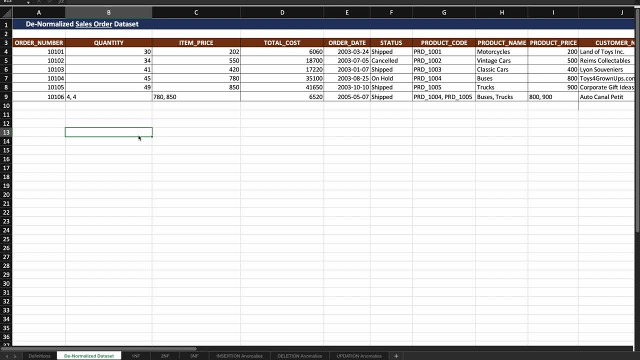 different type of data is bundled together into a single file or a single table, And that is exactly what we have. Okay, once you look at this data set, once you understand this, then you will realize why do I call it denormalized. Okay, now let's first try to understand this data set. what? 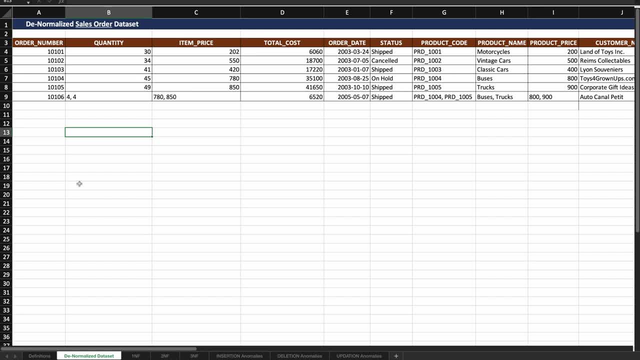 does it actually have? We will try to normalize it step by step. Okay, So this is a sales order data set basically has information about all the different sales order that has happened. So the first column is an order number, basically the ID for or a number for your order. then there is a quantity number of items. 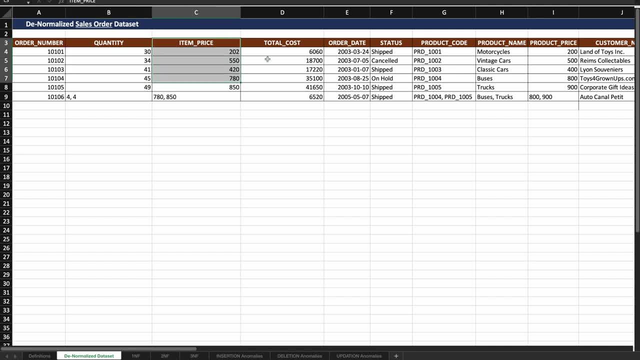 that was sold as part of that particular order, the price of each item, the total cost of the order, the order date and the status of the order. Okay, then we have information about the product, the product which was actually sold as part of this order. So the product code is mentioned here. 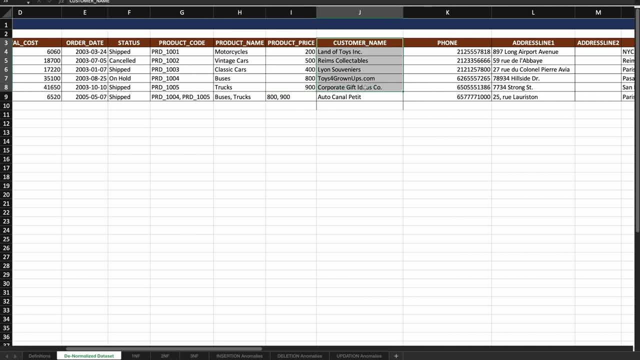 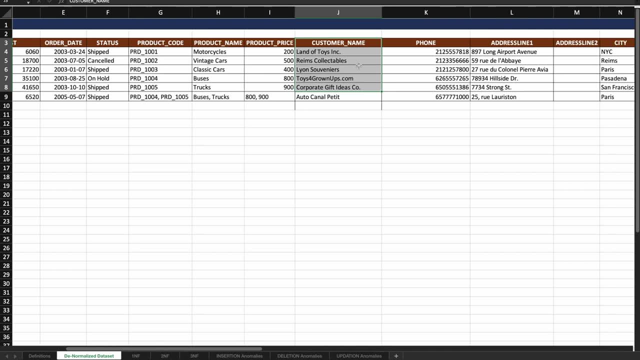 these two columns. then we have the customer information, the customer who actually purchased this order. Now, you can see that these are not individual customer. these are corporate customers, right? So this is some companies And there is also information about these companies. 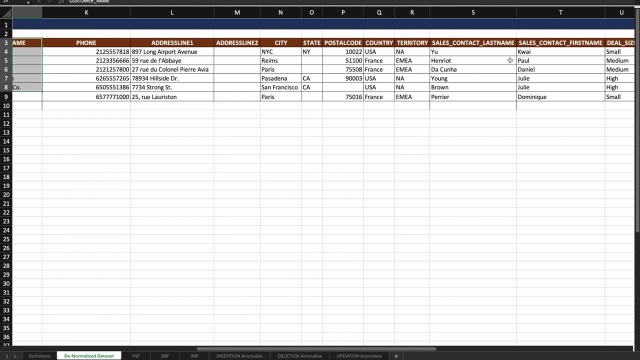 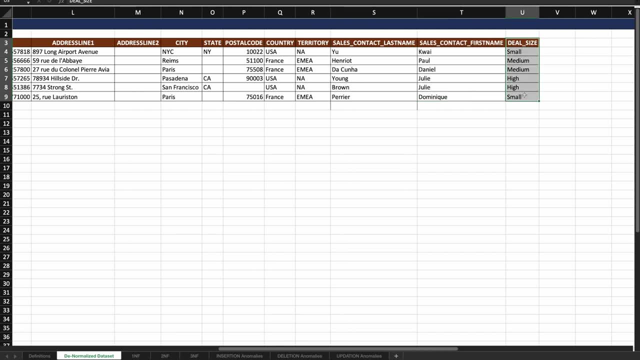 their phone number, their address, their city, postal code, etc. And finally, we also have a couple of columns about the sales agent who are responsible for this order, And at the end we have the deal. size basically indicates how big this particular order was right. So this is. 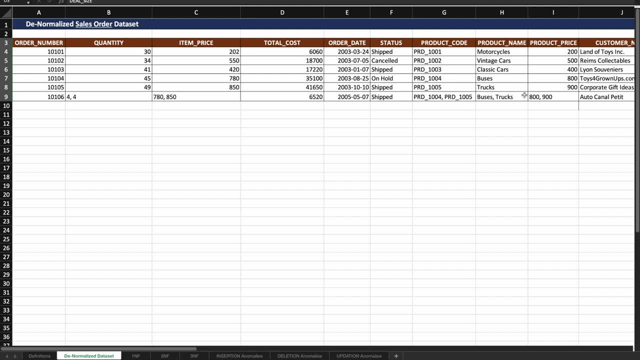 a very complex data set. It's not a very complex data set. I have actually reduced some of the columns just to keep it short and meaningful for this video. Okay, Now let's say you went into a company, your manager gives you this file, tells you that, hey, whatever your name is, maybe let's 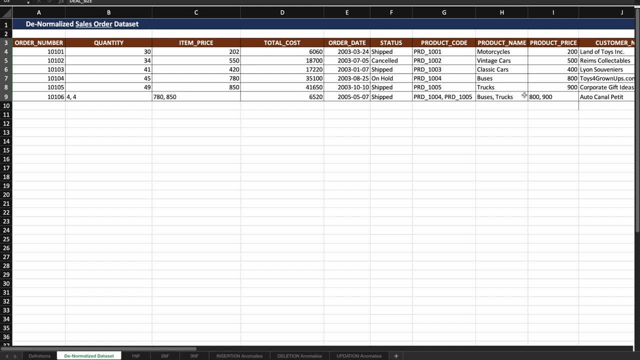 say your name is David. okay, hey, David, I want you to normalize this data set and you can create a new database And make sure that, when you create it, you normalize that database as per this particular data set. Okay, so what will you do? So, as I told you, there is no magic button that you 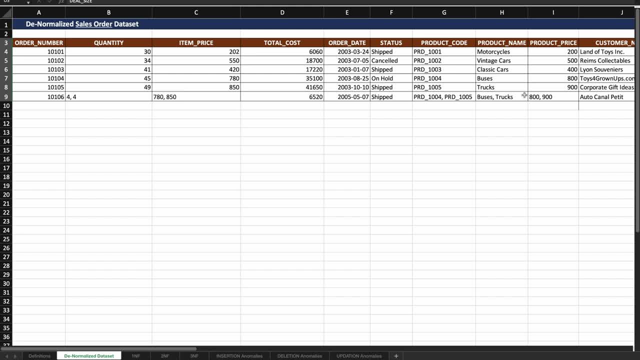 just click and your database will completely get lost So you can create a new database, normalize. you need to follow step by step process. you need to follow each level of normalization to normalize your database right, And that is exactly what we will do Now. the very 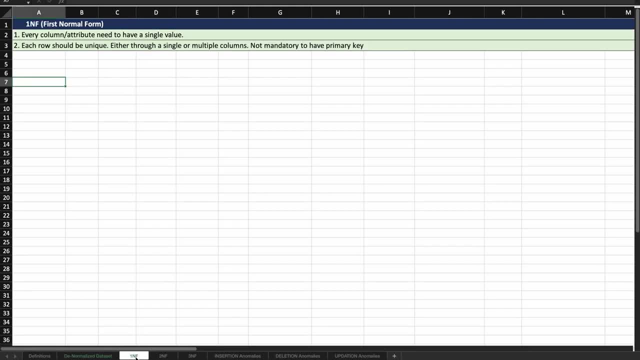 first step in normalization is to make our database satisfy the first normal form. Now, as part of first normal form, we can see that there are two rules that we will need to follow. the rule number one is that every column or attribute, basically they are the same attribute. 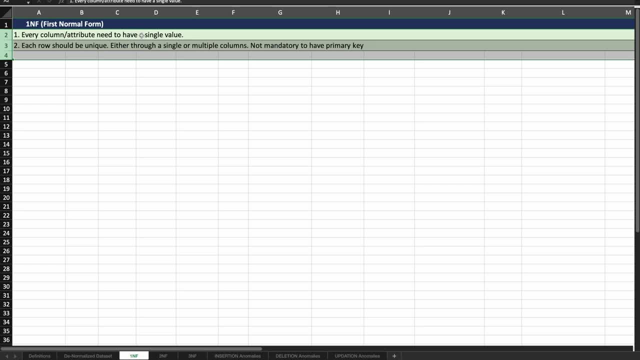 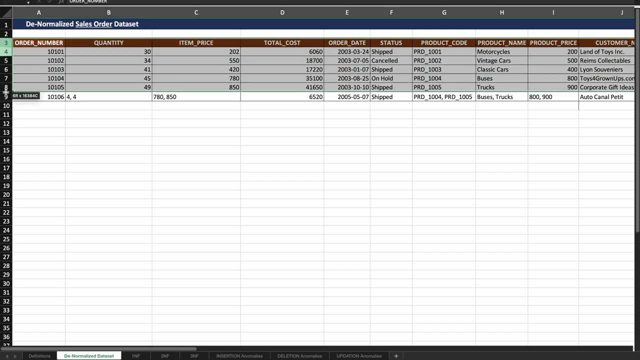 or column basically means the same: every column needs to have a single value. Okay, that's the rule number one. Okay, Now, if I go back to my data set here and let me just copy this data set and move it to this next sheet so that we can make it normalized step by step. 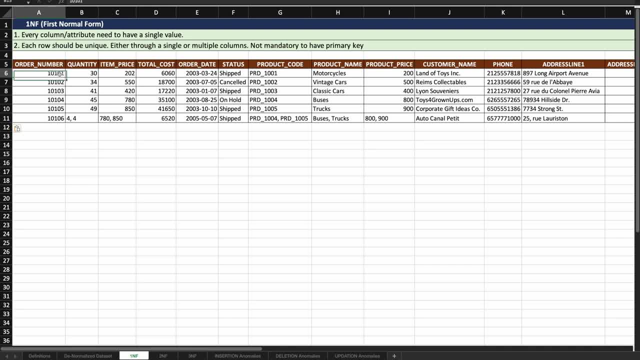 So I'll just put it here. Okay, And now, if I look at this data set, is there any column in this data set which does not satisfy rule number one? let's look at that rule says every column should have one single value. Now I can see that almost every, in fact every column here has one single value. 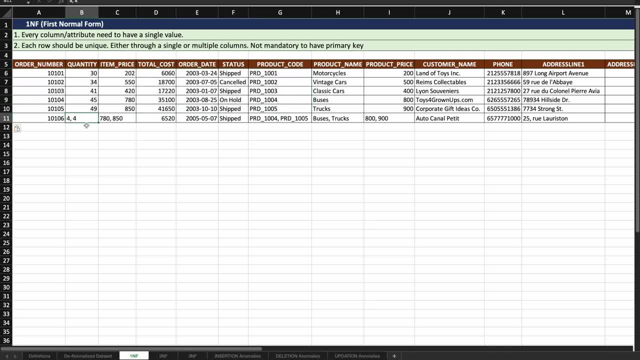 except for some of the columns in the last record. Here I can see that there is a comma by comma separated values. So there are two values here, there is two values here, And then you can see: here also there are two different product codes mentioned, here also two different product names. 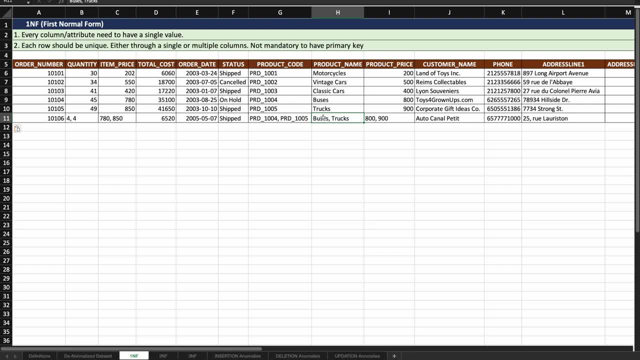 mentioned right. So what this means is basically: this was like there was a single customer who purchased two different items, but the company basically provided just a single invoice order. Okay, So in the single invoice or in the single order statement, they have basically merged the 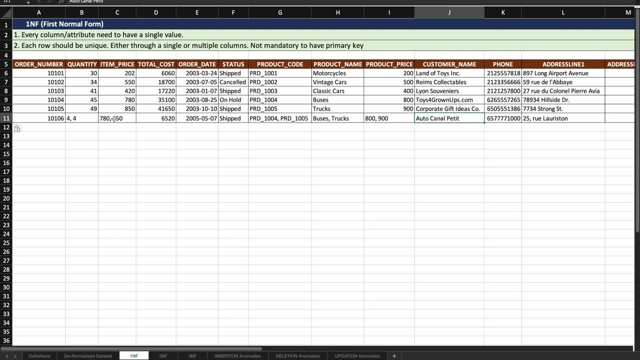 details of two different items. Ideally this should not happen, right? So don't treat this to be something like when you're going to a supermarket, when you purchase 10 different items and you will get just one bill or invoice when you go- let's say you go with your brother. 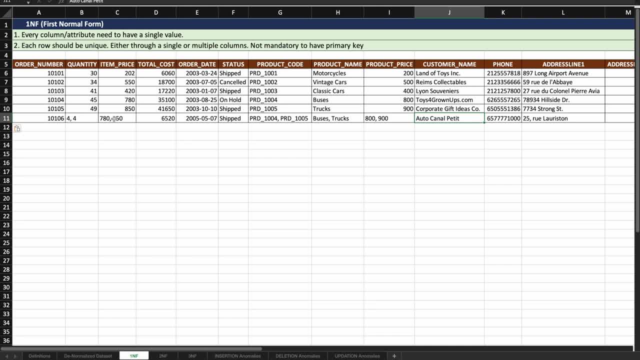 and you're buying a car, you would definitely be given two different invoices, right? they would be two different, cars would be built separately, And here we are talking about big products, right, as you can see here, right? So ideally, this is not correct, right? We cannot be having two different. 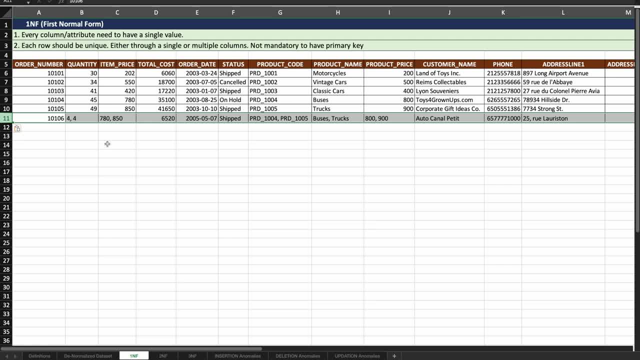 items build together into a single order right. Ideally, this should have been split into two different columns, And this also does not satisfy the first normal form. each column should have one single value, And that is exactly what we will need to do first. So first of all, even before, 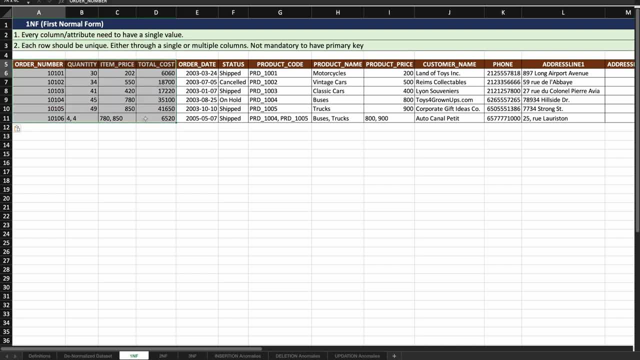 we look at the rule number two. let's just try to change this data set such that it will satisfy the rule number one, So we will need to split these multiple values in the column into. each value should have its own record. Okay, so what I do is I'll copy this whole thing and I'll paste it here. 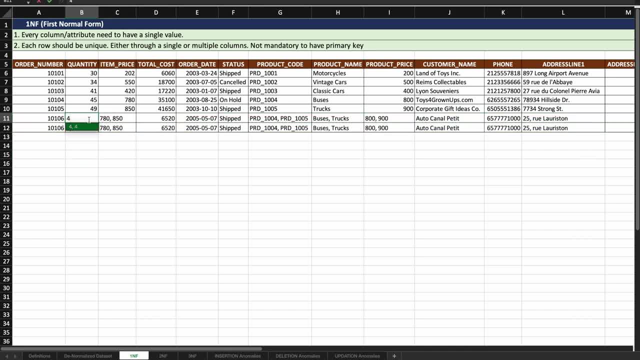 and I'll remove one of the values here. So I'll put one four here and I'll put another four here, okay, And then again the same thing: 780 and 850.. So 780 and 850, right, And then okay, this one. 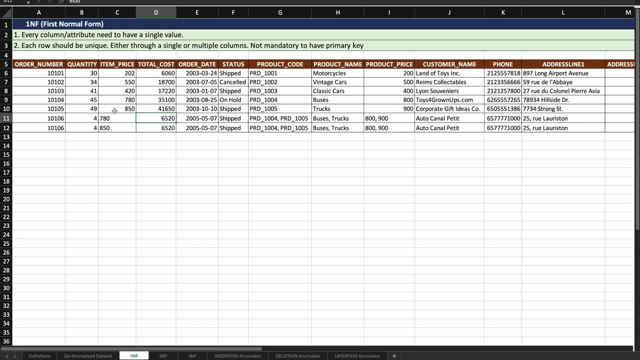 I need to multiply four into 780, because it's a total cost or quantity into the item of each price of each item. So I think this one will be 3120.. And this one should probably be 3400.. Okay, and then the products. So let me just keep the first product in the first line and the second 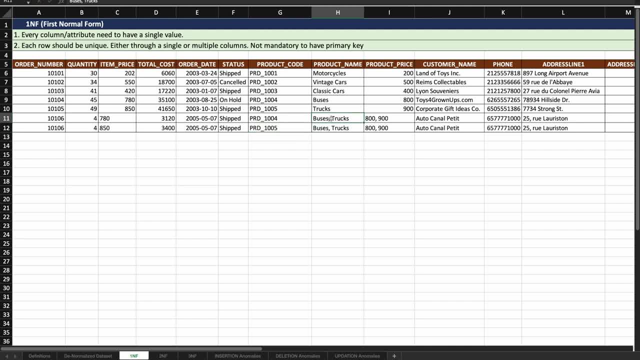 product. I'll move it to the second line here, Okay. And the same thing with the product name. buses will be at the top and the trucks will be my last order, Okay, And the same thing with the price: 800 and 900.. Right, Hopefully. I think that's all. I have basically split all the double. 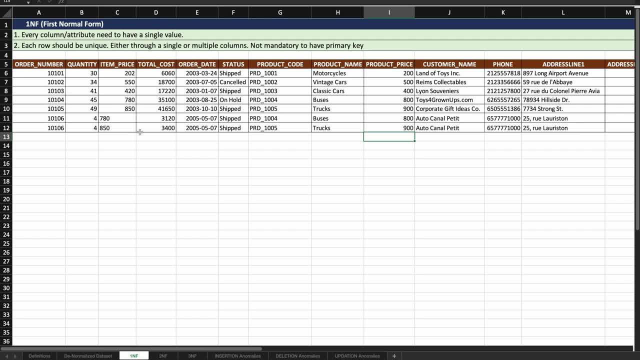 valued attributes or columns in now having single columns. okay, only single values in each column. just that one of the record has increased, right? So imagine if you had three values here, then you had to basically split it into three records. Okay, I hope that makes sense. So now I can say that. and if I go, 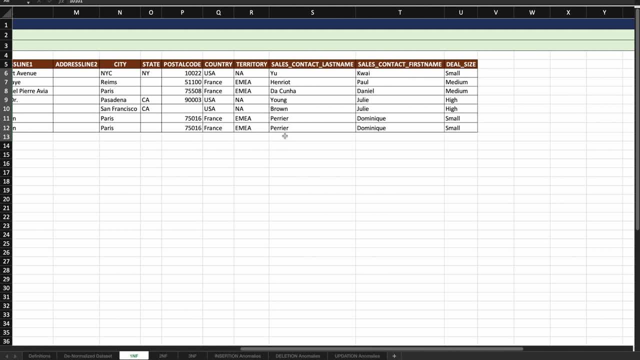 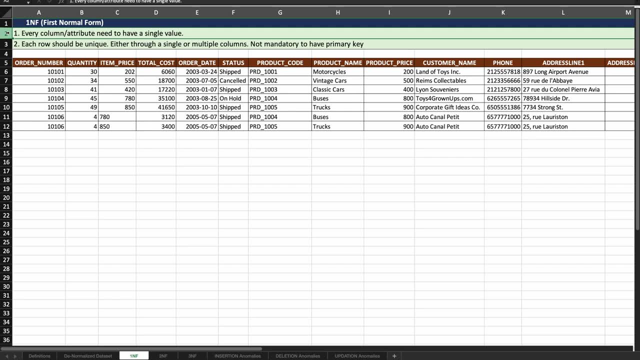 to the right, I will see that there are no columns where there are multiple values in a single column. Okay, So I can say that this whole data set now satisfies the first rule of my first normal form. Right Now, let's look at the second rule. The second rule states that each row should be: 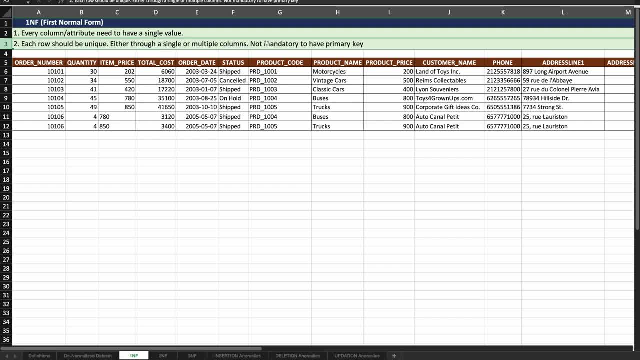 unique, okay, either through a single or multiple columns, and it is not mandatory to have primary key. Okay, So they're saying it's not mandatory to have primary key. if there was a primary key, then well and good, But if it is not, it's still okay. 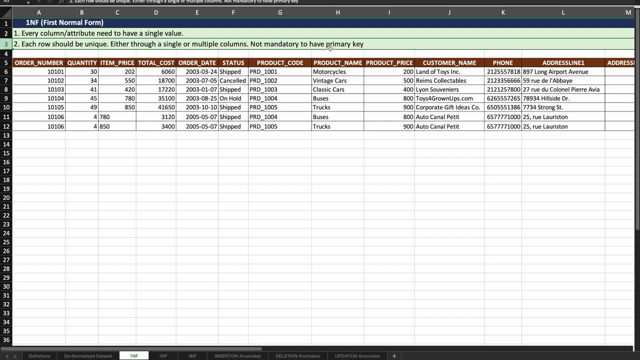 just make sure that you have unique records. How do I see if these are unique records? So, first of all, my very first five records. I can tell them that they are unique. Why? Because the order number itself is unique. So every record will be unique. definitely right, But when it comes to 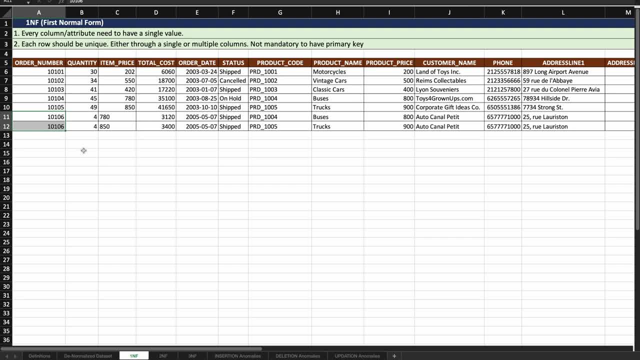 the last record or the last two records, I can see that both these records are sharing the same order number. Okay, So I can see that both these records are sharing the same order number, Right, But then each of this order is for a different product. So if I could combine this? 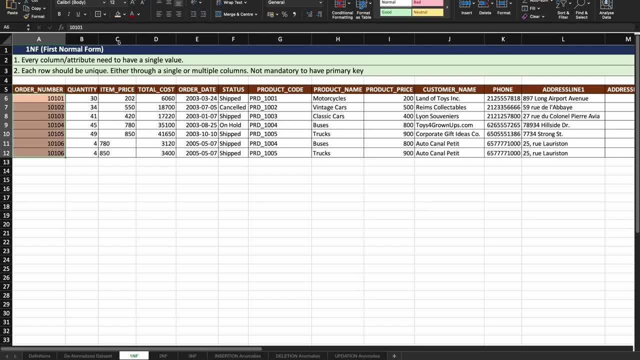 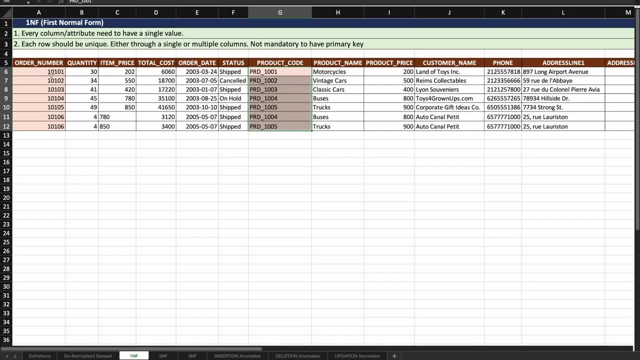 column. so let's say, if I could combine this column. or let's say, let me maybe color it like this. And let's say, if I combine this column, so the combination of these two columns, order number and product code, is basically unique, right? Because the last two records here, if you just 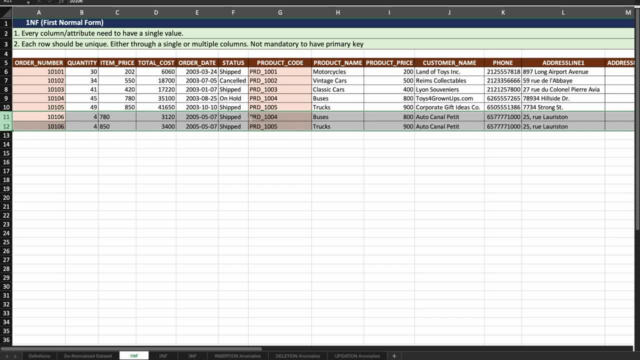 carefully see, the order number is 10106.. But it is two different products, So the records are unique, even though it's the same customer. these records are unique when I take the combination of order number and product code. Okay, So basically for rule number two. this is already satisfying rule number two. 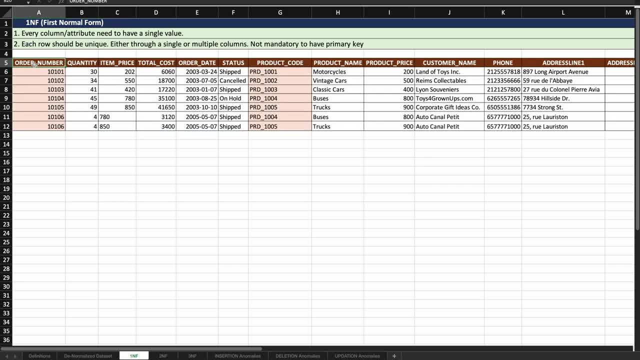 I basically have nothing to do here, So I can say that this data set now is in first normal form. Okay, so my first level of normalization is done. Now let's move on to the second level. Hey, there, are you still watching the video? If yes, then make sure that you have clicked. 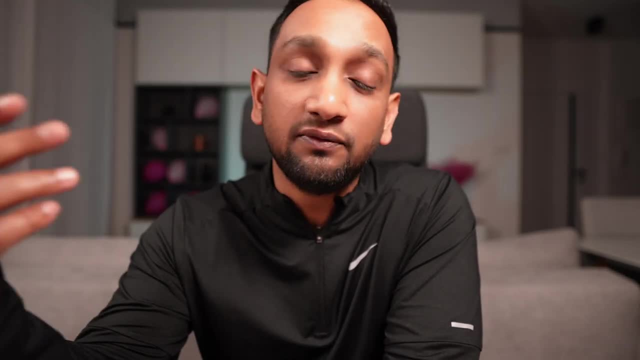 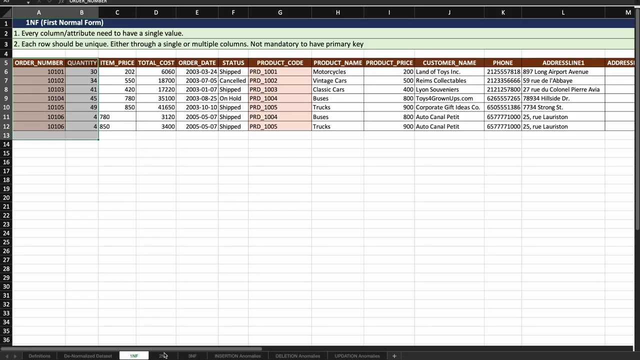 on the like button and you have subscribed to the channel to watch more such videos. Make sure you subscribe Definitely. leave your feedback in the comments below. I would love to read them. Thank you so much, And let's continue with the video Now as part of the 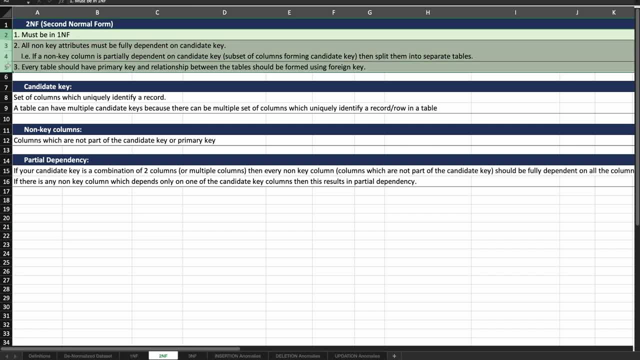 second normal form. there are three different rules that we will need to follow. Okay, now for now, just try to ignore these definitions. I will explain this when I come to that. But if you see, the first rule of second normal form basically tells that it has to be in first normal form. 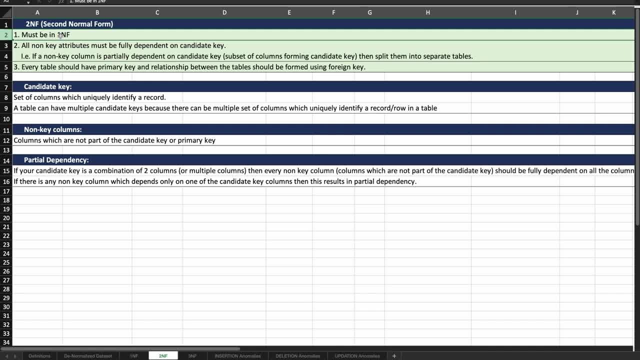 So even before you come to level two of normalization has to be satisfied. that is, first normal form should be satisfied before you can basically try to satisfy the second normal form. that's rule number one. the second rule is that all non-key attributes must be fully dependent on candidate key right now, even before we proceed further, or 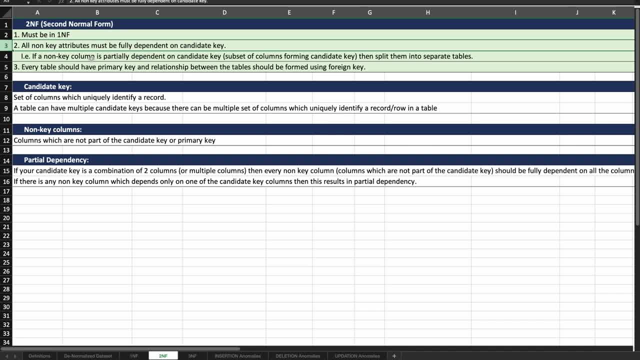 read further. let us first understand what do we mean by candidate key? okay, now i have these definitions here just so that i could save time in. if i had to type them here it would take more time. so i have all, all of them ready here, okay, so basically, candidate key means that these are: 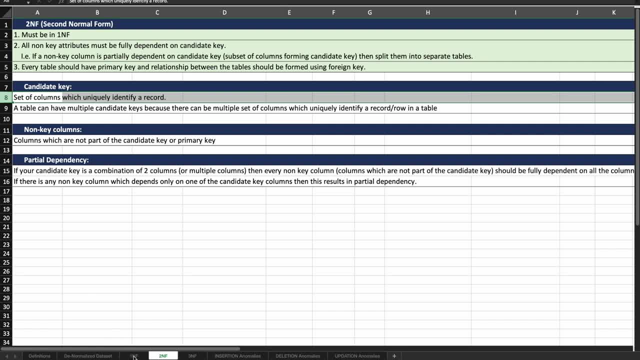 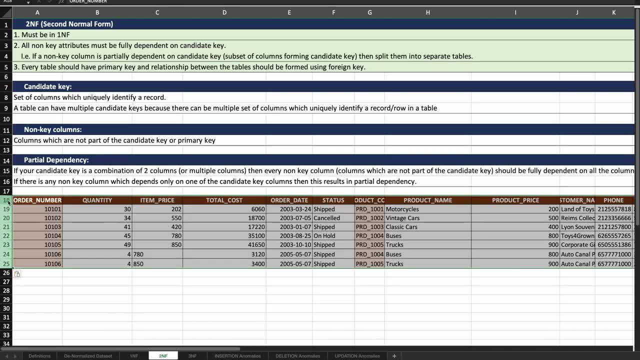 the set of columns which will uniquely identify a record. for example, let's say, i'm going to copy this data set and put it into our next tab. okay, just so that it becomes easier for us to understand. okay, so this is the data set which is now satisfying the first normal form. right now, what? 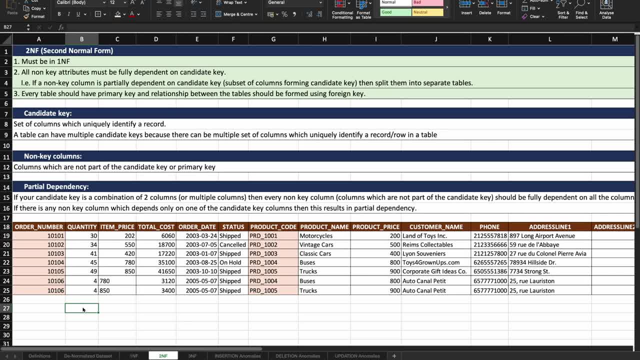 exactly do we mean by candidate key, right? so candidate key is basically the set of columns that will uniquely, you know, identify a record. In our case, in this particular data set, I can easily tell, as we discussed before, the combination of order number and product code is always unique as per this data set, right? So? 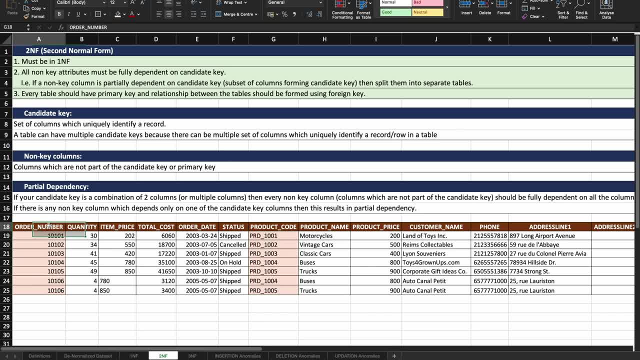 in our case the candidate key becomes the combination of order number and product code. So basically in our case the candidate key is order number plus product code. okay, So I am saying plus. probably in SQL we can say concatenate. okay, Now this is basically what my candidate key 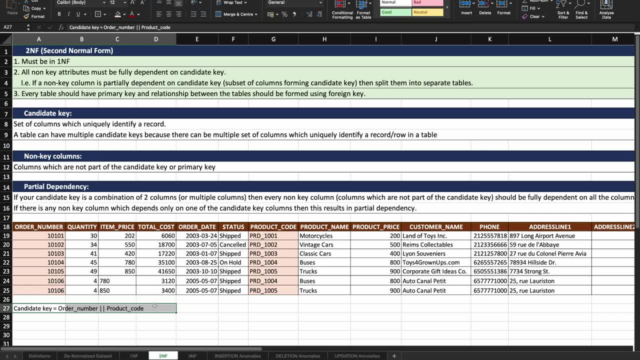 for this particular data set. okay, So okay. and one more thing to remember is a table can have multiple candidate keys. okay. Now, this candidate key is not a primary key, It is a secondary key. So it is a secondary key, So it is a secondary key. So 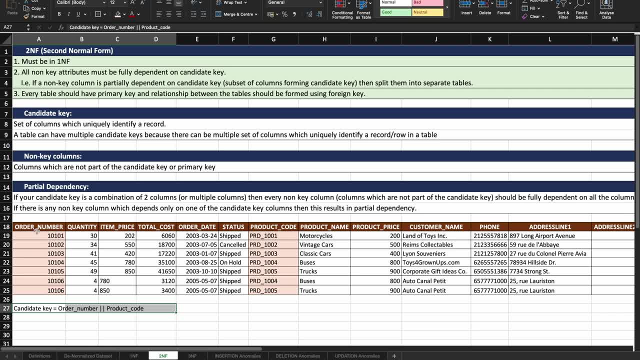 I have not created a primary key for this data set, So primary key is different from a candidate key. okay, And you can have multiple candidate key because there can be multiple columns or multiple set of columns in your data set which might form a unique record. right, So any combination. 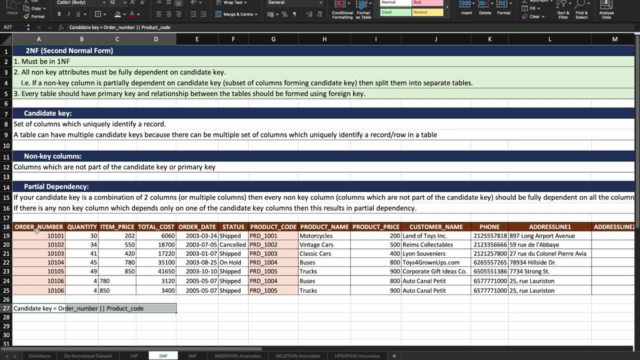 of column which forms unique record. we can call them as candidate key. okay, So remember that. And the other thing that you need to remember is what do you mean by non-key attributes? So basically, any other column which is not part of the candidate key or the primary key. 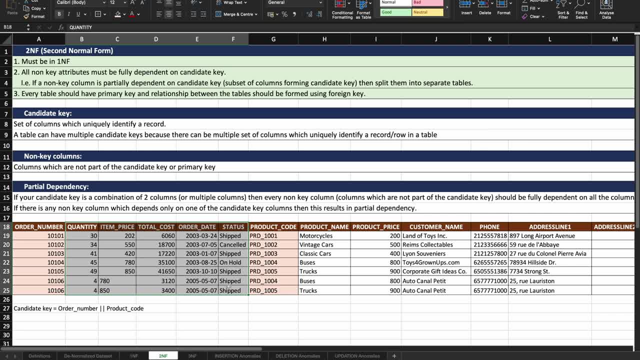 we treat them as non-key column. okay, I hope these two concepts are clear. Now let us try to understand the rule number two. So basically, the rule number two of the second normal form states that all non-key attributes must be fully dependent on the candidate key. okay, What exactly does that? 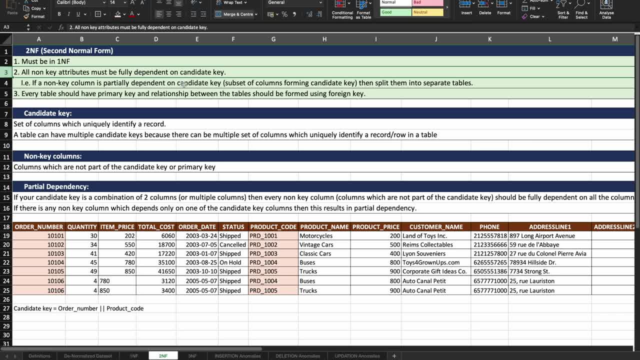 mean. That is, if a non-key column is partially dependent on a candidate key, that is the subset of columns forming the candidate key- then split them into separate tables. Let me try to explain that in simple words. okay, So all non-key columns should be fully dependent on candidate key. So, for example, these columns here: 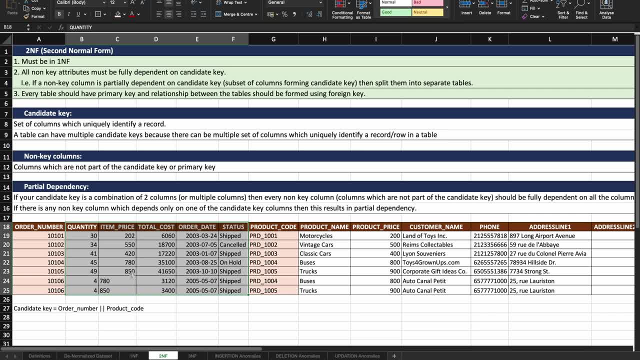 are. I can say that these are my non-key columns right Now. the quantity item, total cost, order number status: these are all the columns which are directly dependent on the order number right, Because each of these values are basically with respect to an order number. With respect to this. 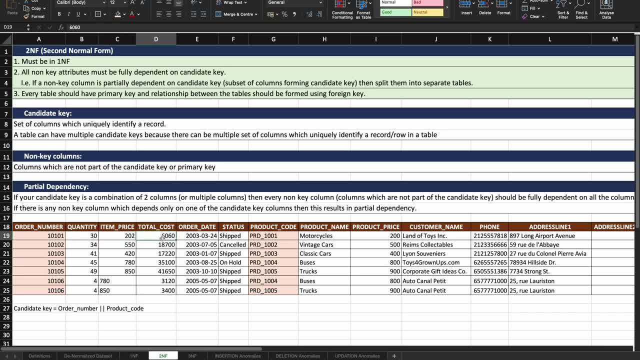 order. this is the quantity, this is the item price, this is the cost, etc. right, So all of these columns are directly dependent or dependent on only on the order number. They have nothing to do with the product code, right? My candidate key is a combination of these two columns, but I have some. 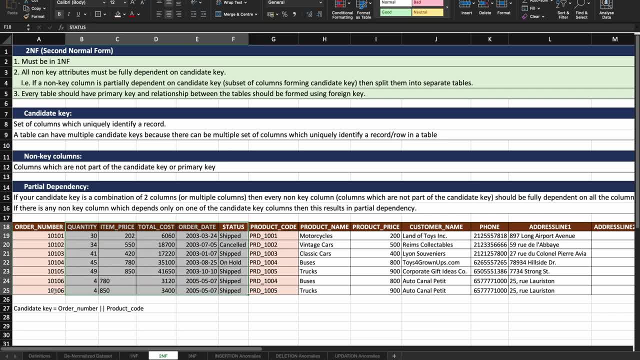 of these non-key columns which are dependent only on one of the columns which is forming the candidate key. So that means these columns are having partial dependency on one of the candidate key columns, right? So this means that these columns here do not satisfy the second normal form. So basically, we will need to split the columns. okay, Now, these are not the. 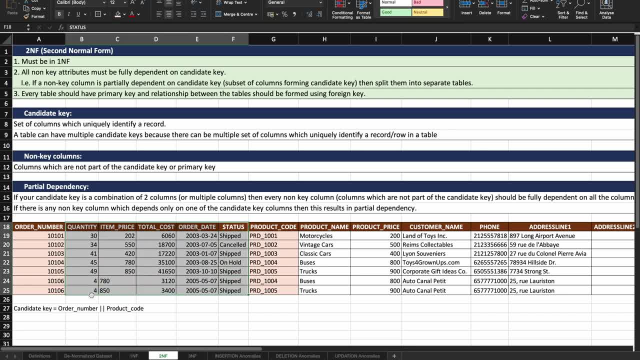 only non-key columns, right? So these columns here definitely does not satisfy the rule 2 of second normal form, So we will need to split them. Similarly, if I look at the product name and product price, these are the columns which are directly linked to the product code. So the name 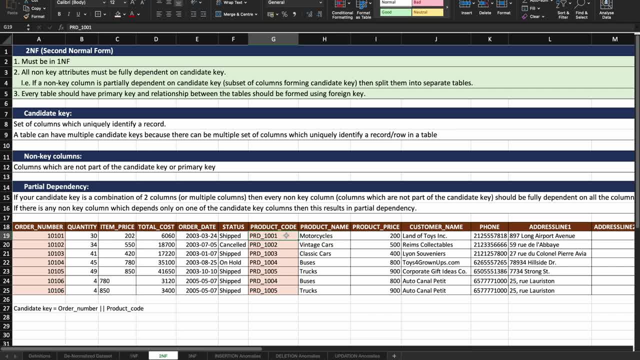 motorcycle is can be represented based on this product code. It has nothing to do with the order right. So this product name and the price has nothing to do with the order. They are only dependent on product code. that is just one of the columns of the candidate key. 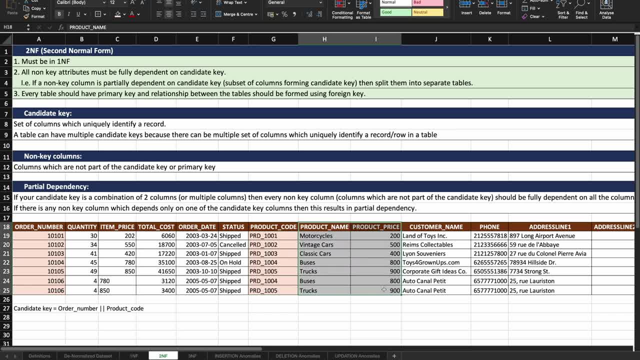 Again, these two non-key columns are partially dependent on one of the candidate key columns, So which will basically not satisfy the second normal form rule. So again, we will need to split these columns right. Similarly, when I look at the customer, So I have the customer name here. 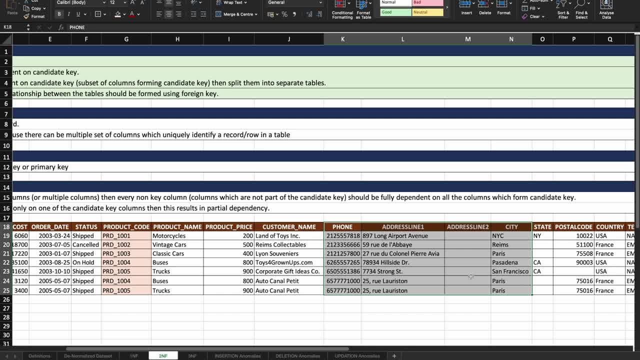 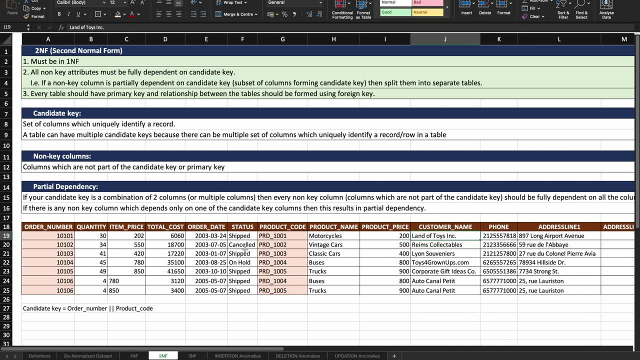 and then I have some other information about the customer: their address, their phone number, etc. Now the phone number, the address and other details about the customer are specific to each customer. They are not specific to an order or specific to a product code, right, 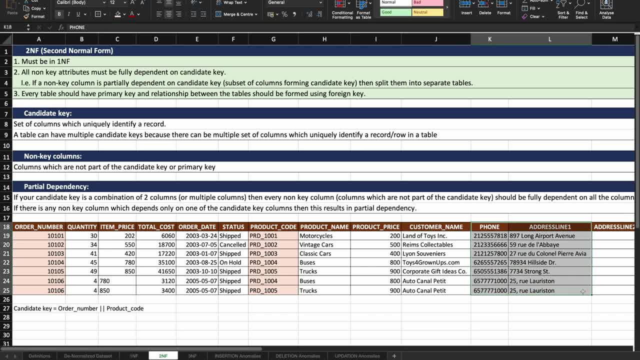 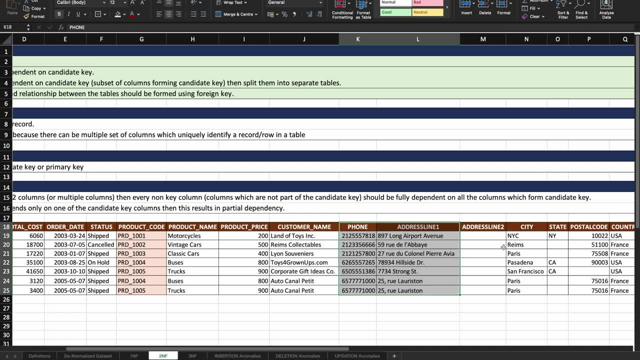 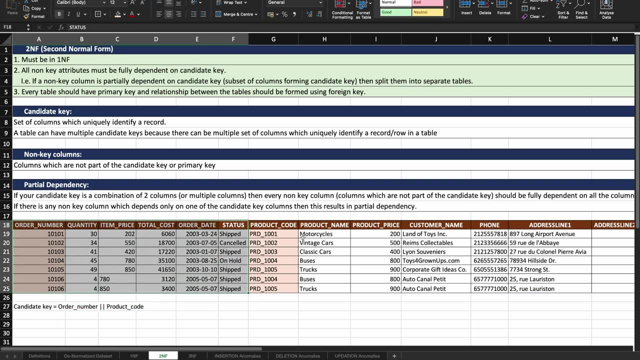 These columns here have basically not dependent on any of the candidate key, So in such cases we again will need to split these columns into a separate table. So this is the first, or basically the second, rule that we will need to satisfy. So basically we will need to have separate tables for all of these orders. We need to have separate tables. 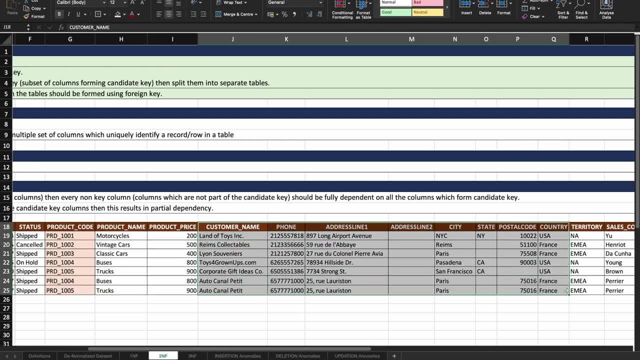 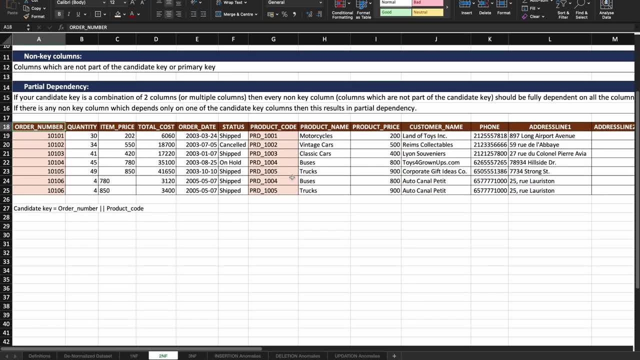 for these products and we need to have separate tables for this customer information, right? So let us try to do that. So what I am going to do is I am going to create an orders table, So maybe I will just keep this as it is and I will just move this. So I will move all of my products into 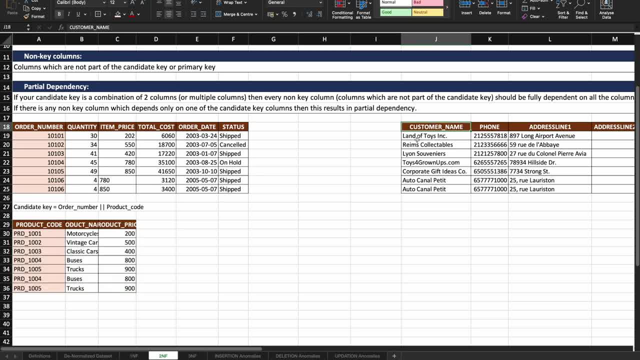 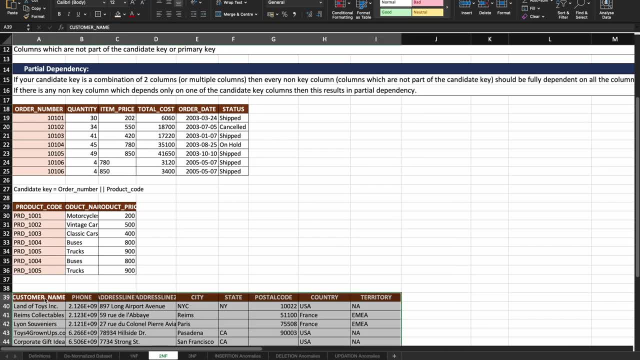 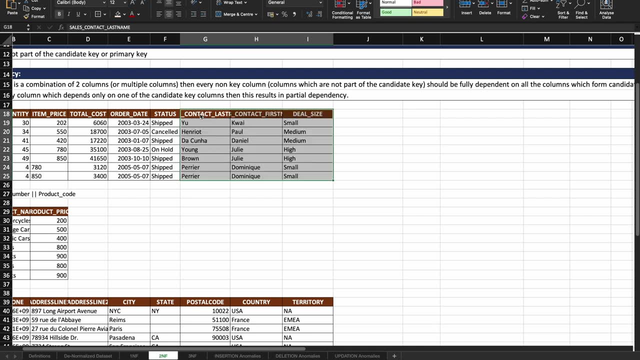 a next table here And then I will move all of my customers into the next table. So I will just cut them from here and let us say I will probably move it here, And then I will just bring the last three columns closer to my orders table here So it becomes easier for you to see. Now, okay, so I think 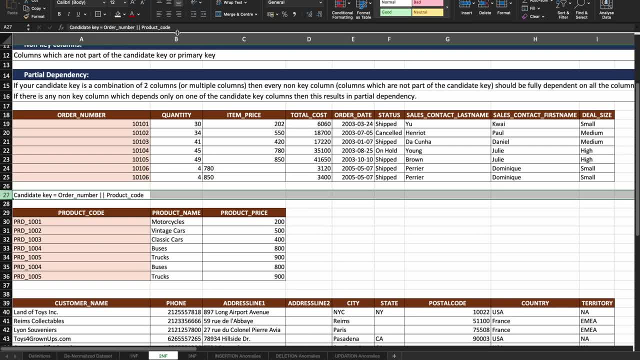 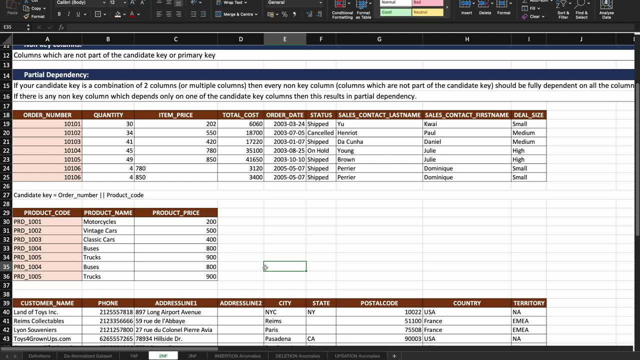 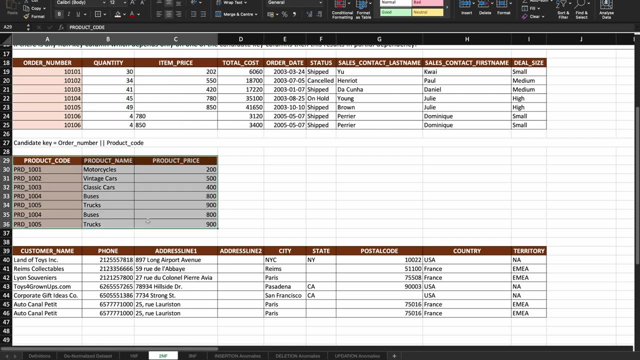 probably this makes sense And let me just merge them so it does not ruin my formatting. Now, okay, so I have basically split my data set into three different tables, as you can see, And I can call this my orders table, this is my products table and this is my customers table. 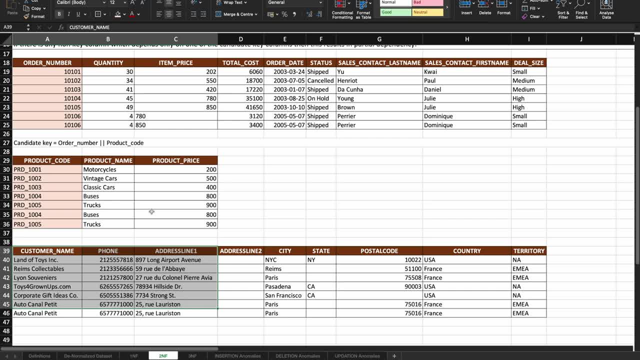 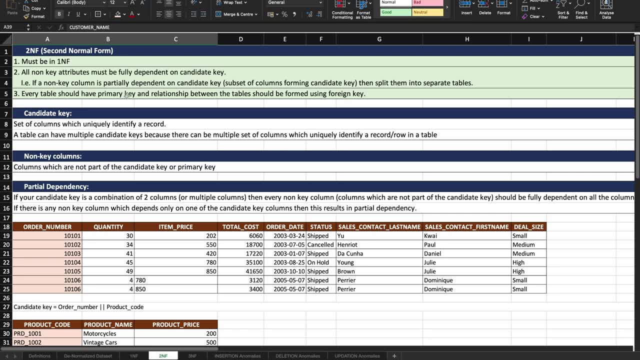 Now, this is the first rule, But this is not the okay. this is the second rule in second normal form, But this is not the only thing. So, once we have basically split them into multiple tables, then we should make sure that every table should have a primary key and 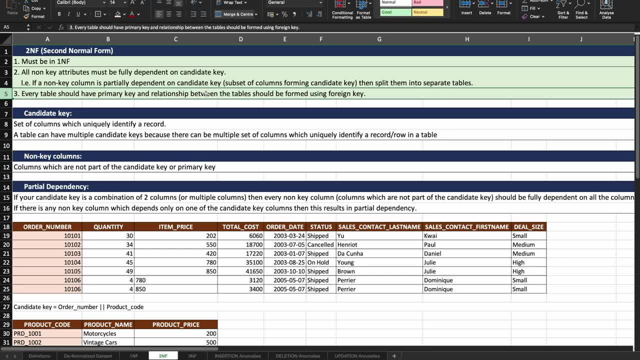 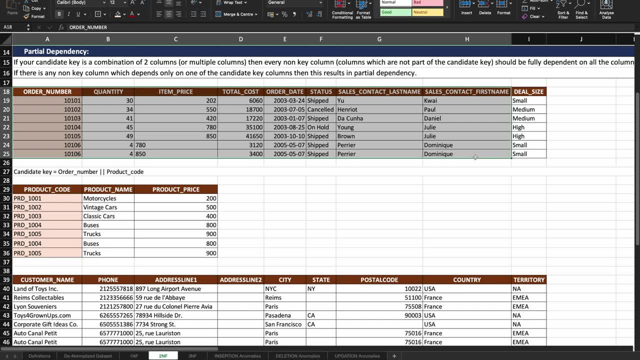 relationship between the tables should be formed using foreign key. So the first thing is we should make sure that every table that we have now split or created needs to have a primary key. So that is my orders table. So this is my orders table. maybe let me just mention that. 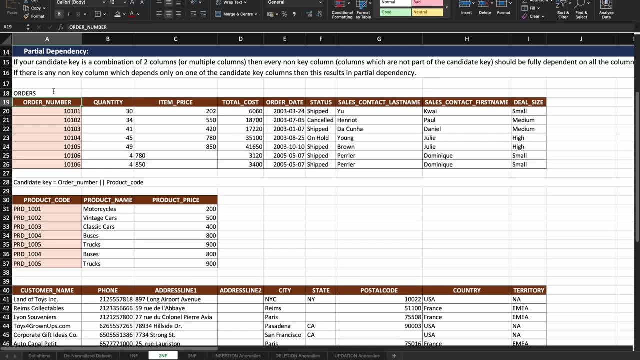 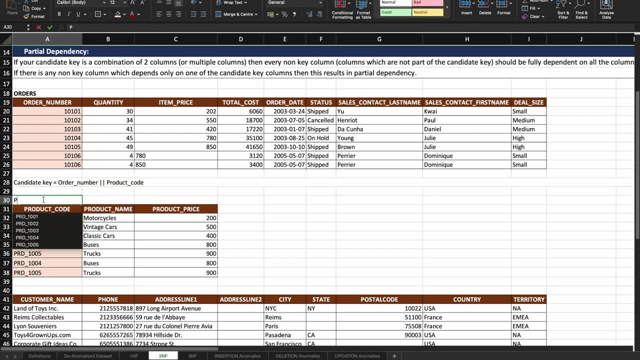 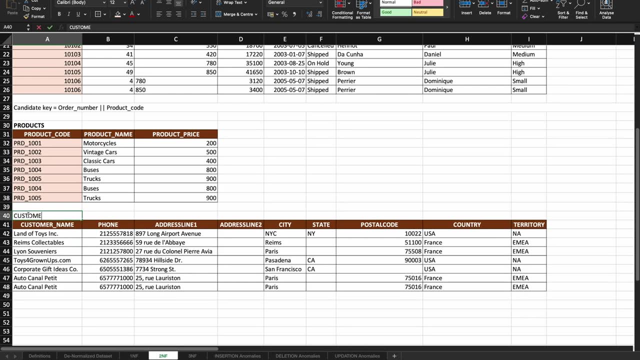 in case, if it confuses anyone. So this is my orders table and this is my products table. So let me just move this here: products table, I'm just giving like a table name, okay, And this is my customers table, okay. So I think that's fine for now. okay, So maybe just to highlight them, I'll 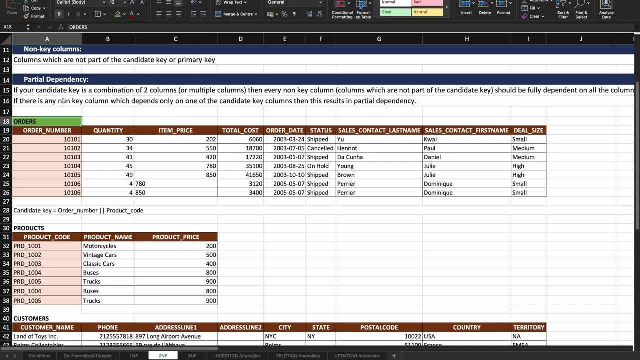 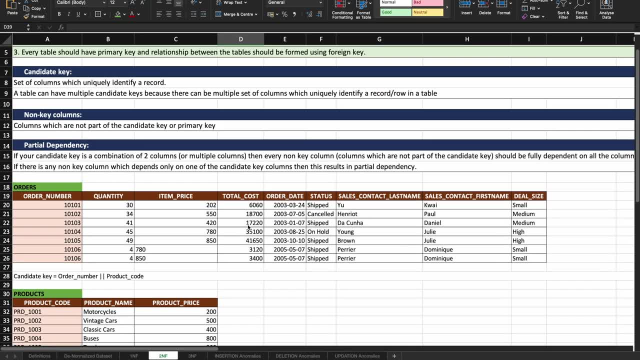 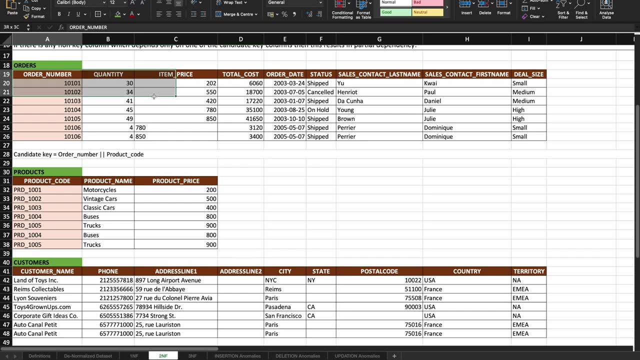 just highlight them in, maybe green, okay, So it just becomes easier to remember. okay, So I have two tables which I have split. Now the next thing is I need to create primary key here, right? So, if I see I do not have any primary key. So I have this order number, but the last two records are: 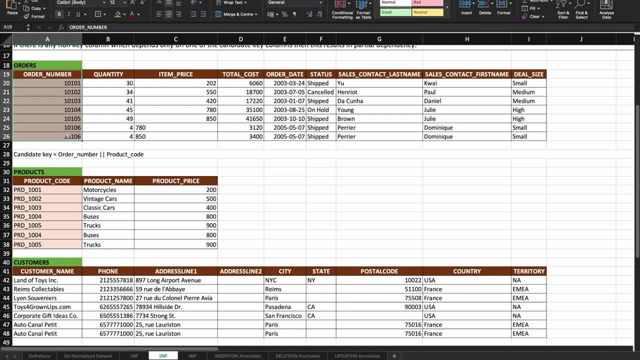 basically having the same order number. So I cannot consider this to be a primary key. So what I'll do, I'll create a new primary key for this table. So I'll just move this to the right. I'll create a new column and I'm going to call it like order id. okay, And here I'll just tell one, two. 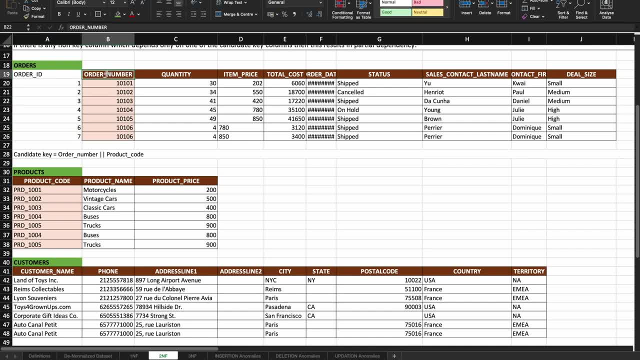 three, four, five, six, seven. okay, So just some standard values, Just to just for the sake of example, and I'll just remove this highlighting of the column because I don't need this as of now. okay, So I have created one of the primary keys for this. 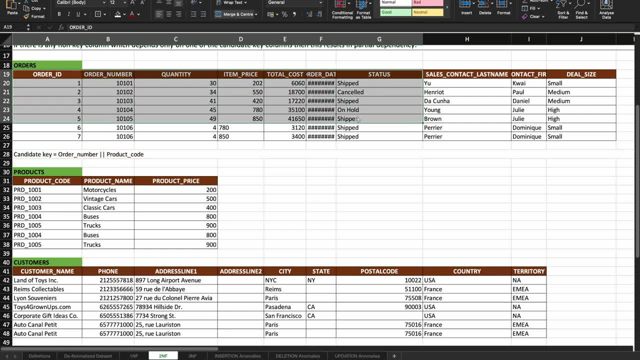 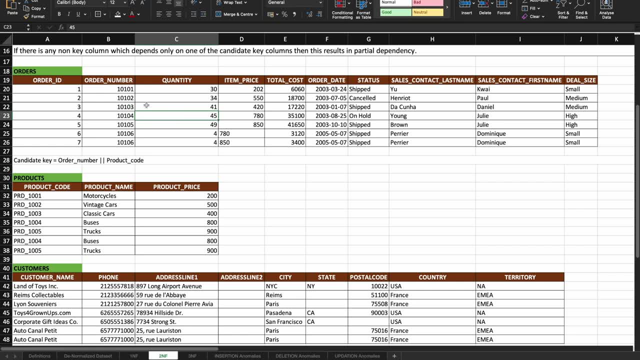 table. that is order number. that is the orders table and I think this looks fine. okay, So if I just format it again, I think this, so my orders table looks fine. there is a primary key. that is fine. The next is product stable. Now for products table. I don't really need to create a primary key. 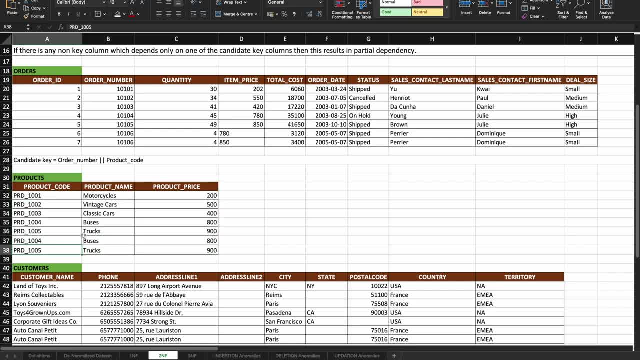 that I have a product code. probably I can use this to be my primary key, but there are certain duplicate records, So these buses and trucks are repeated twice, right? So, first and foremost, since it's a separate table and I don't need to store these products multiple times in this separate 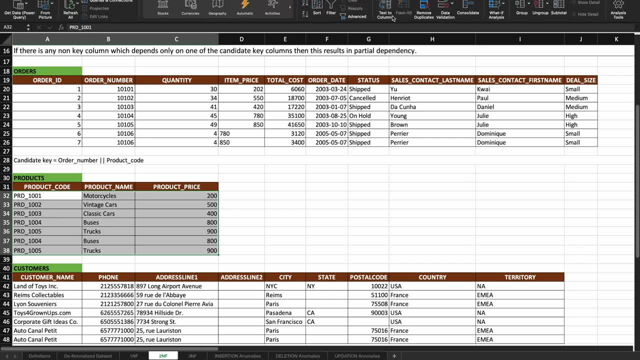 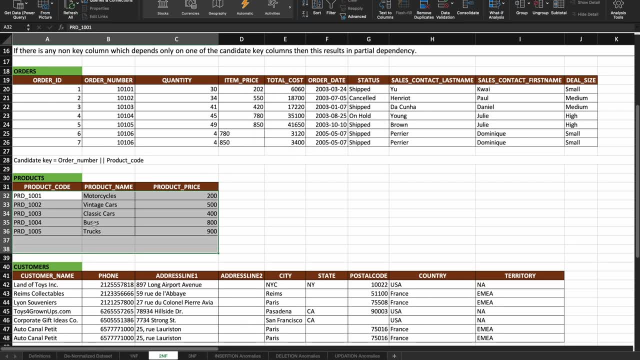 table. I will just remove the duplicate records. okay, So I'll just go to the excel functionality of remove duplicates and I'll just click on that and you can see that two duplicate values found and removed. So now I have unique products and I can treat my product code itself to be my 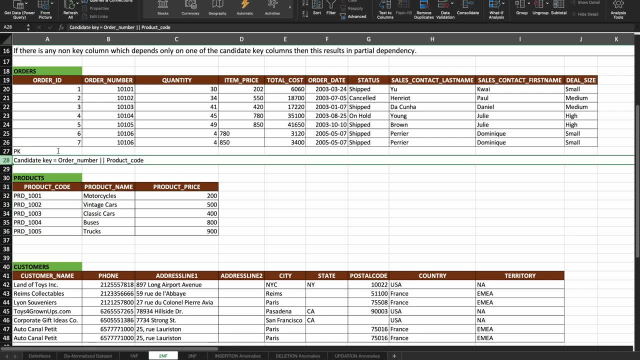 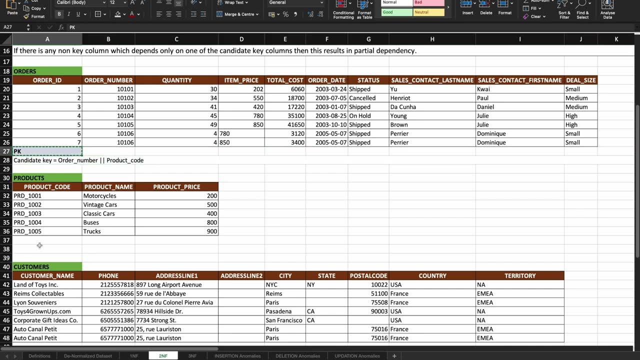 primary key. So here I'm just going to call: this is my primary key column, okay, and let this, let me just highlight this separately- So let's say, or maybe something lighter: okay, So this is my primary key column. okay, and this will be my primary key column in the products table, that is. 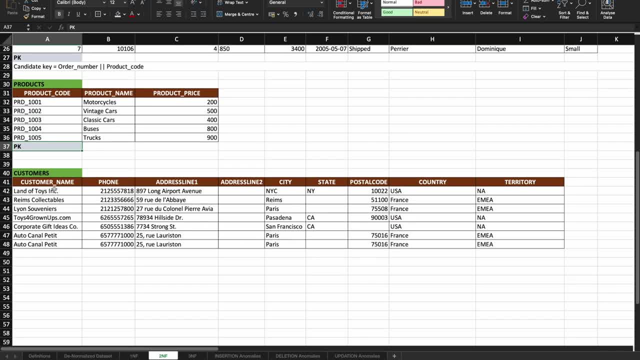 product code. and then, when it comes to my customers table, you can see that again, I do not have any primary key here. right? The customer name cannot be treated like primary key. One more thing is: I can see that this customer here is repeated twice. I don't need to store the. 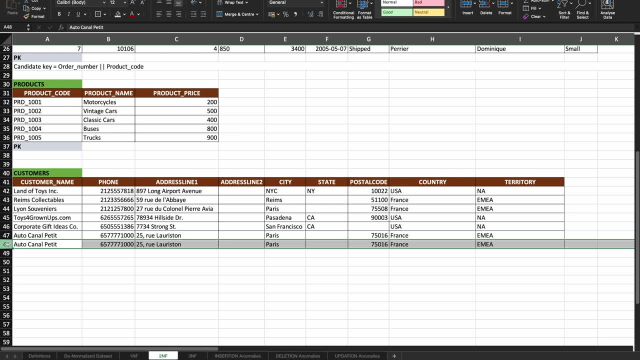 same customer information multiple times in the customers table. I can remove one of them. So again, I'll just select entire thing and I will try to basically remove the duplicate records, okay? So I'll just say remove duplicates and you can see one of the customers is removed, okay. 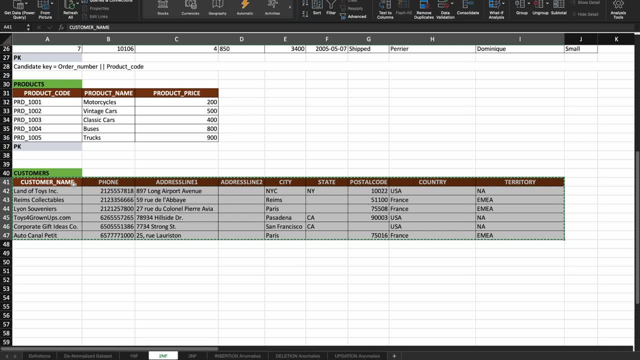 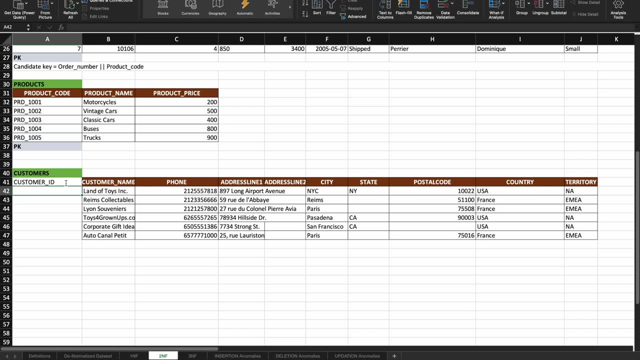 Now the next thing is to create a primary key. I do not want to consider the customer name as a primary key, So what I'll do is I'll create a new column here, which I'm going to name Like customer id, and this is going to be my primary key. So I'm just going to name. 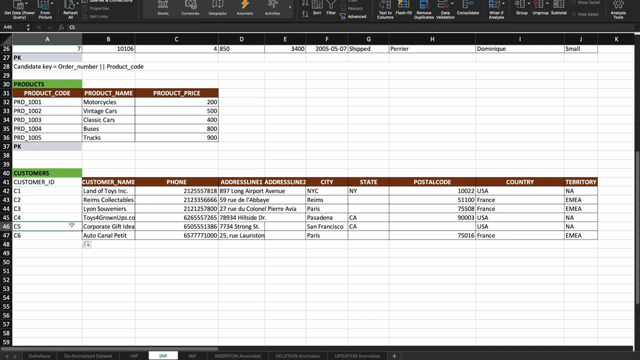 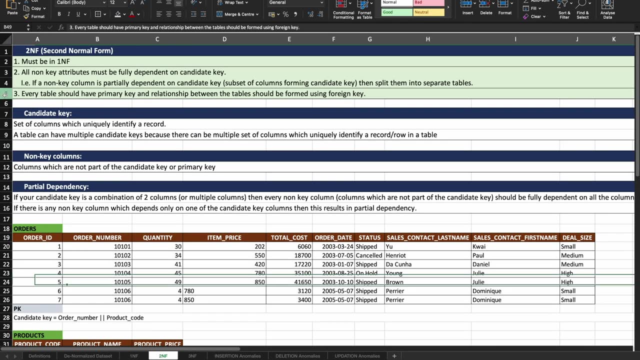 give values like c1 until I think c6. okay, and I'll use the same formatting for this and I'll put it here. okay, So now I think I can say that all my three tables are having primary keys. So that is fine. So one part of my rule number three is satisfied. The last part is that: 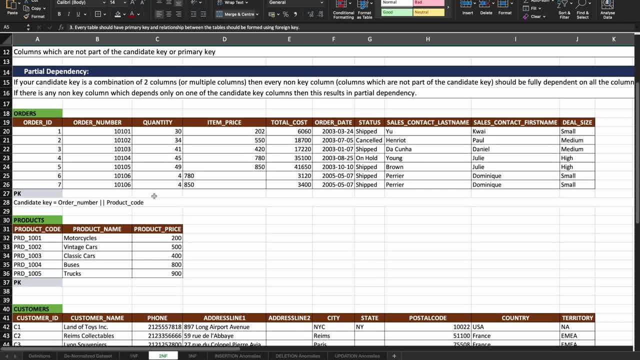 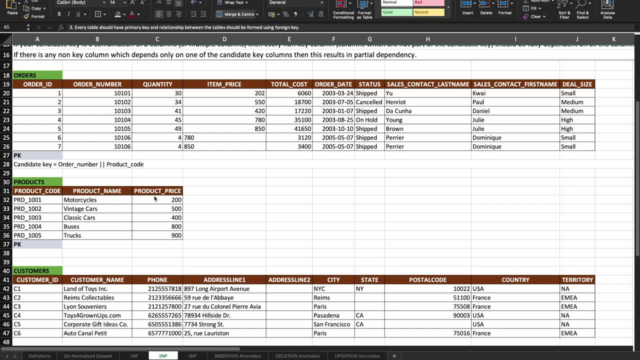 I need to build relationship between these three tables. okay, Now here is a very important point I want you guys to remember, and that is: you can normalize your database in multiple different ways. There is no hard set rule that this is exactly how you should normalize your database. 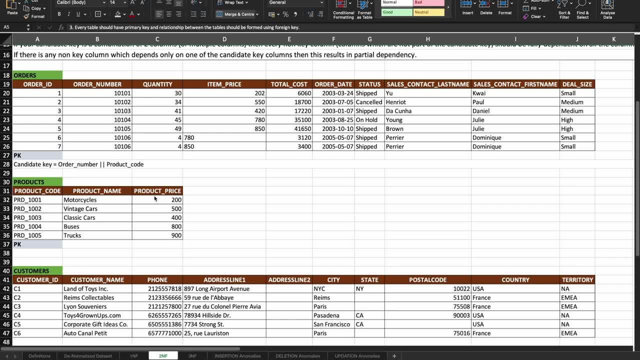 There is nothing like that. okay, It depends on you, your project, your requirement, your company, your teammates and so many different factors how you would like to normalize it. For example, in this particular case, I could satisfy the rule three of this second normal form in two different. 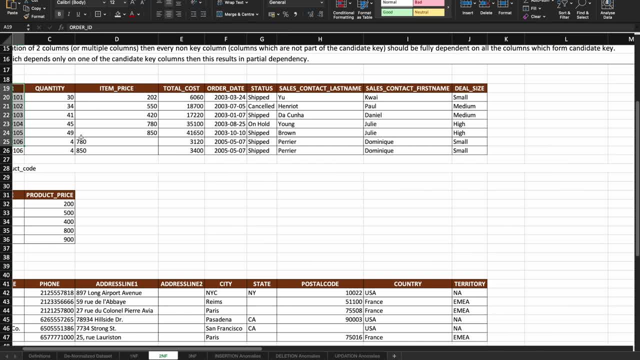 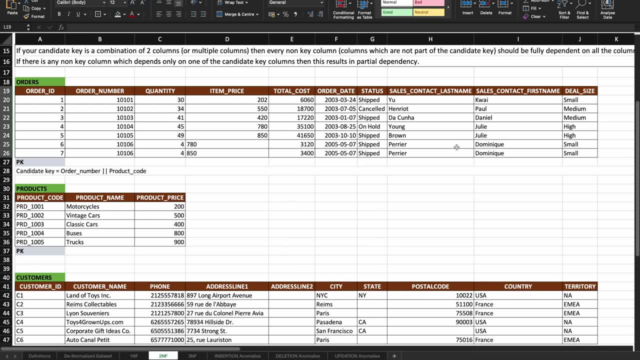 ways. One, what I could do is, in my orders table itself, I could add a last column here telling this is a product code here and a customer id here, and that would still satisfy my second normal form. or what I could do is I could create a new table, something like a relationships table. So what I'll 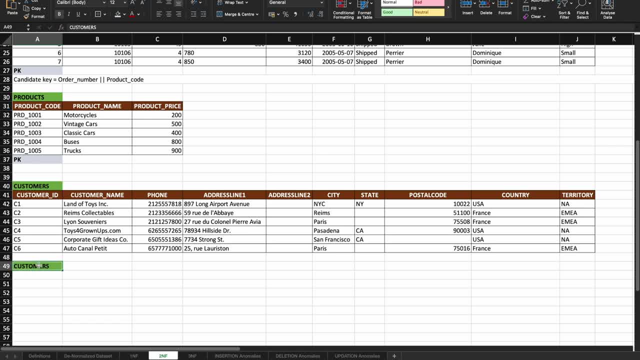 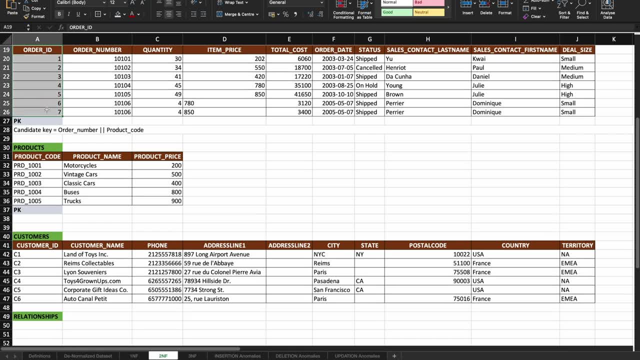 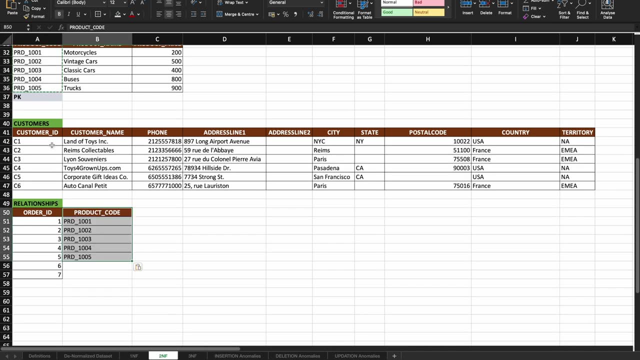 do is I'll create a relationships table- and I'm just going to call it like relationships- where I'm going to have my order number, my product code and my customer id. okay, So I'll have my order number, then I'll copy my product code here, okay, and then I'll copy. 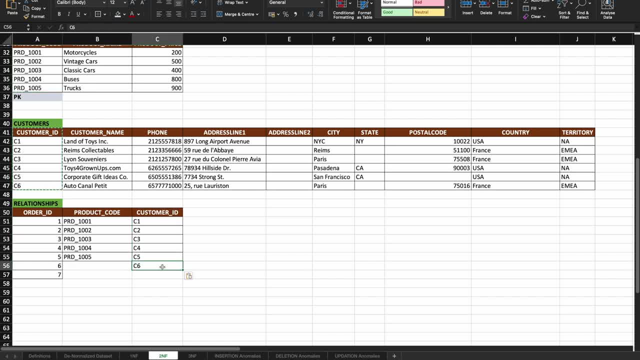 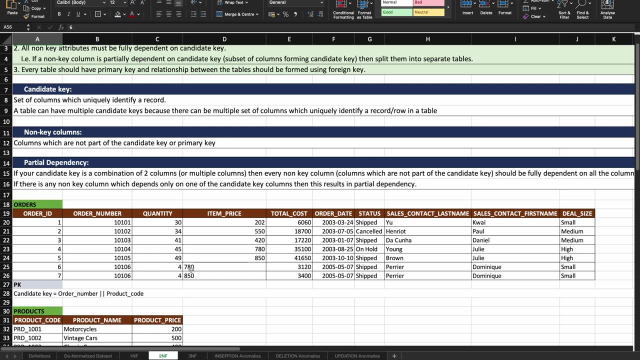 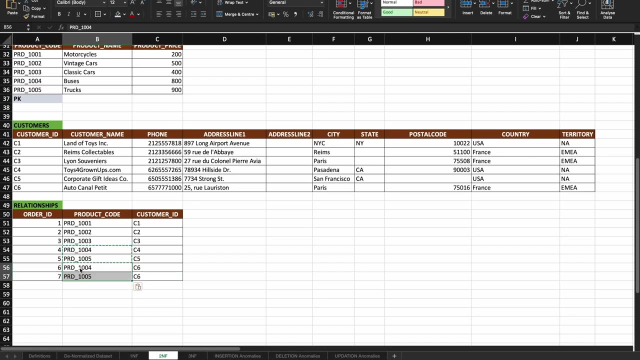 my customer id. okay, Now I know the last two orders belong to the same customer, so I'll paste it here. and I know the last two orders also belonged to this product, that is, I think it was buses and trucks. So what I'll do? I'll just copy this. okay, I am aware of the data, so I am just 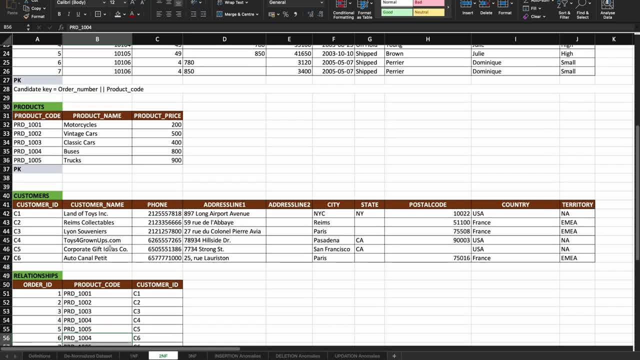 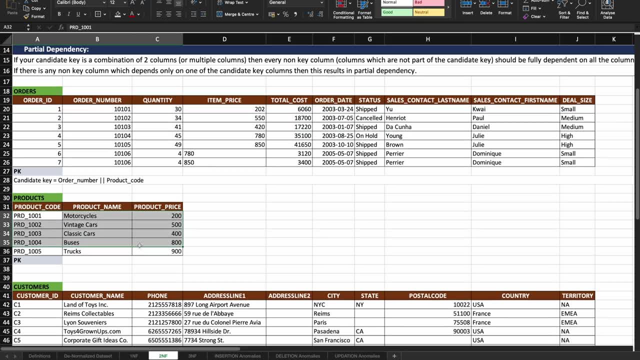 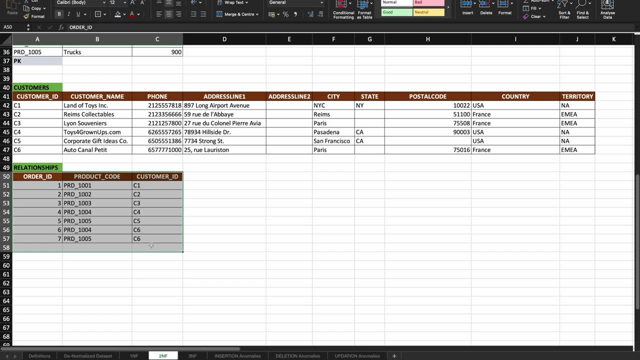 doing it quickly, okay. So basically, what I have done is, instead of adding these two columns at the end of the orders table, I kept the orders table as it is. I kept the product table as it is, customer's table as it is, and I just added a new table where I just have a relationship between: 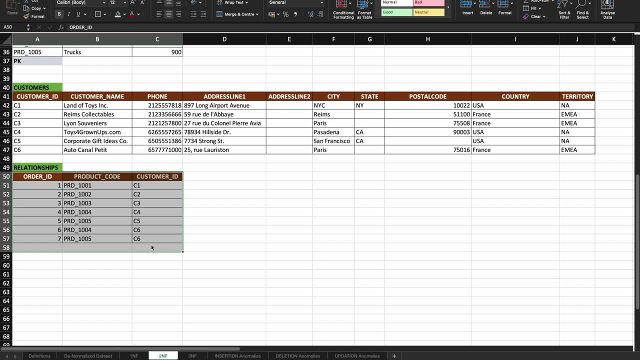 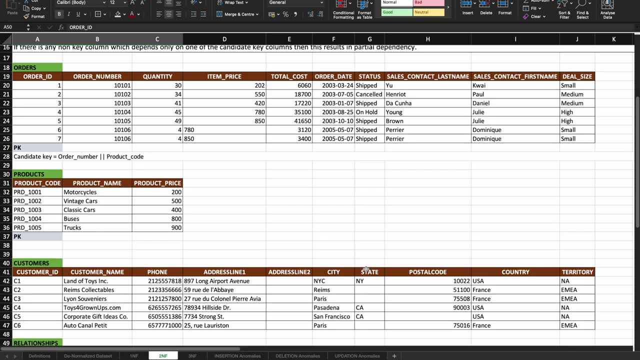 my products, customers and the orders table. okay, So this is completely up to you, your project, how you would like to normalize it. both are right, whether you add these columns to the end of this table or you create a new table, both are right. okay, So I'm just following this. I hope this is. 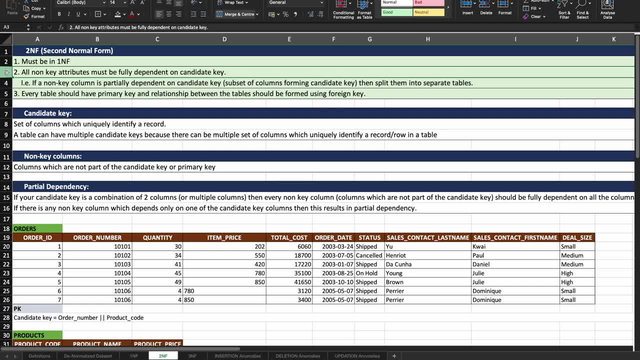 clear. now I can see that my second normal form, this whole data set that I have created, is now satisfying my second normal form. Now I can see that my second normal form, this whole data set that I have created, is now satisfying my second normal form. 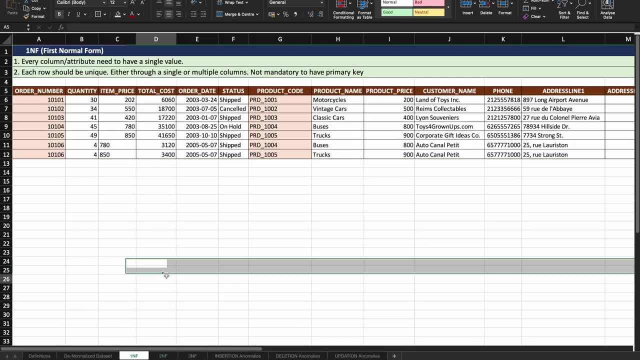 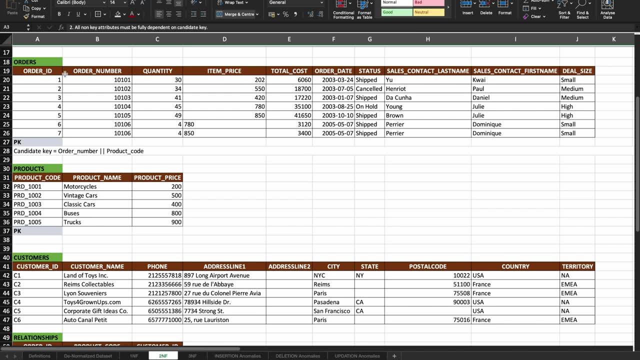 The only thing that you need to remember is when I had first normal form, I just had one table, but when I came to second normal form, I basically have four tables. there is a separate table for orders, separate table for products, separate table for customers, and then there is 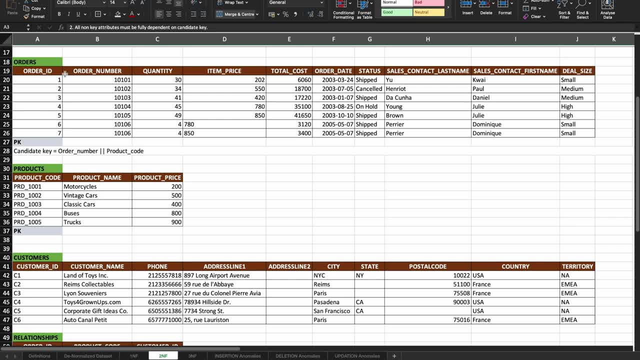 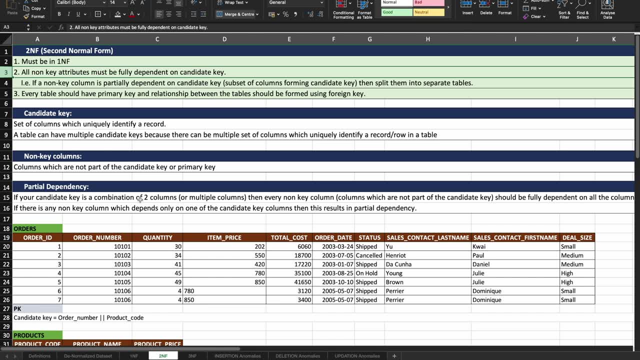 a relationship table which basically has the linkages or relationship between the other three tables. So I hope this is clear. now let's try to normalize our database further such that it will satisfy the third normal form. okay Now if I go into my third normal form, but before that let's. 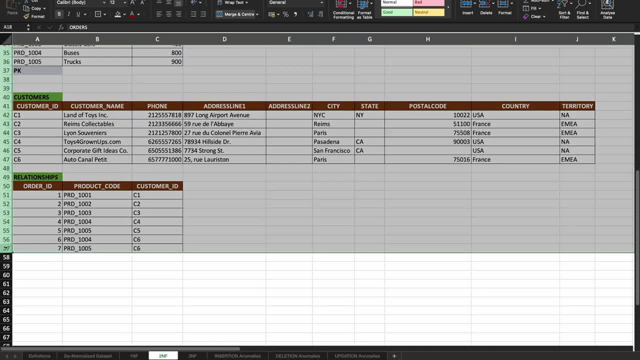 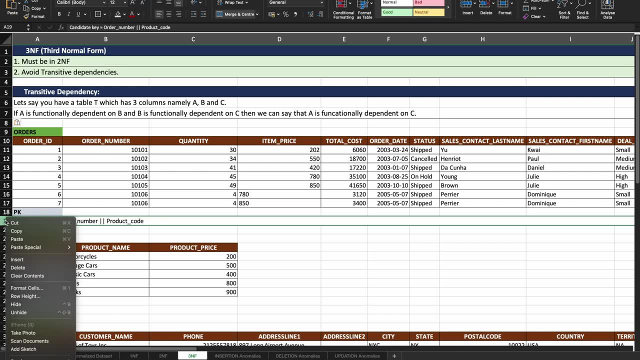 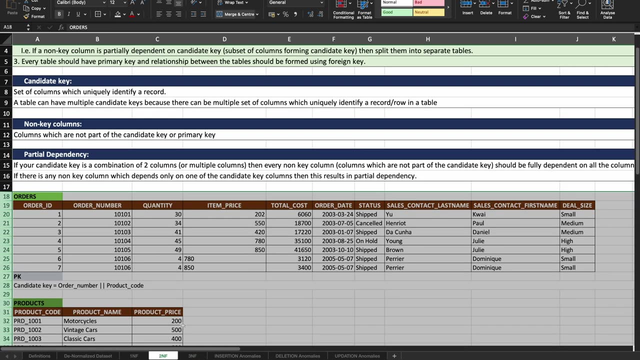 me copy all of this, okay, all of these four tables that I have already created, and I'll just move it into my third normal form here, okay, and I'll remove this, this thing, I don't need it here, okay. So, basically, I just copied the normalized data set as per second normal form into this. 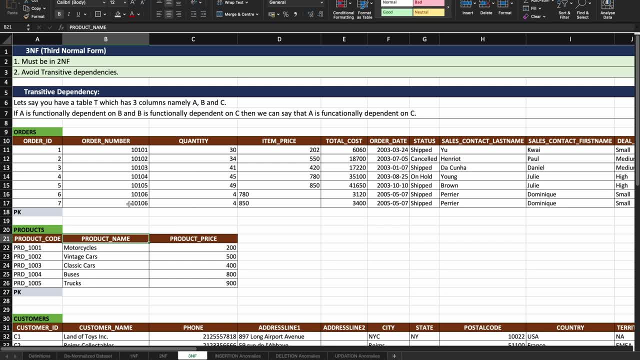 particular tab so that we can make our changes on this data set. okay, So, as per the third normal form, if your database needs to satisfy third normal form, first of all it has to be in the second normal form, or it has to be in the second normal form, or it has to be in the third normal form. 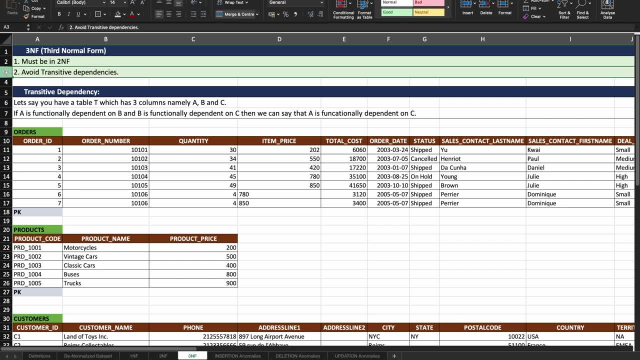 That's rule number one. and the rule number two is it should avoid transitive dependency. So if your database or data set is having any transitive dependencies, then you should split such columns which are causing the transitive dependency. Now, first of all, what do you mean by transitive? 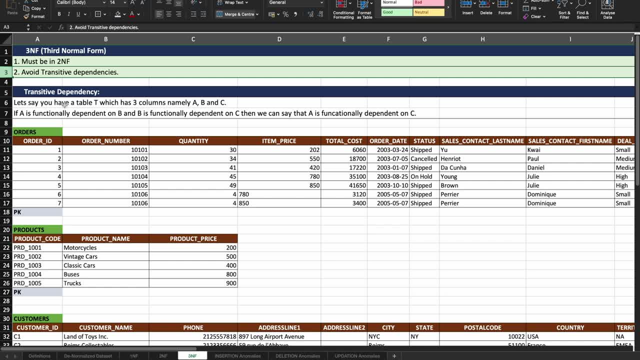 dependency right. So imagine that you have a table by the name t and it has three columns- a, b and c- and let's say your column a is functionally dependent on b and b is functionally dependent on c. Then we can say that if you have a column a and b are functionally dependent on c, then we can. 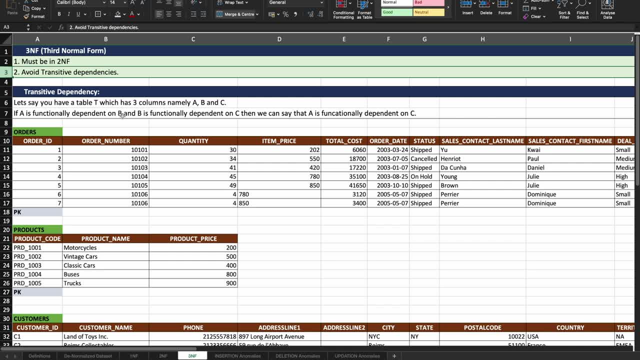 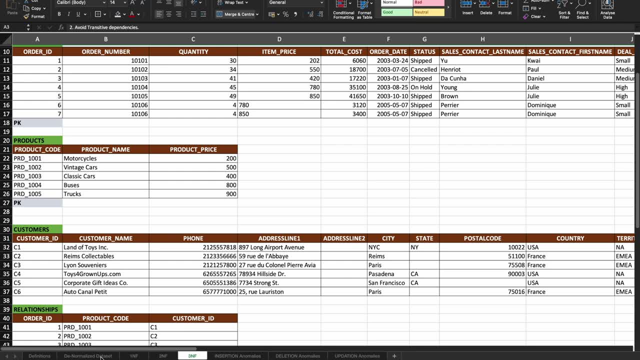 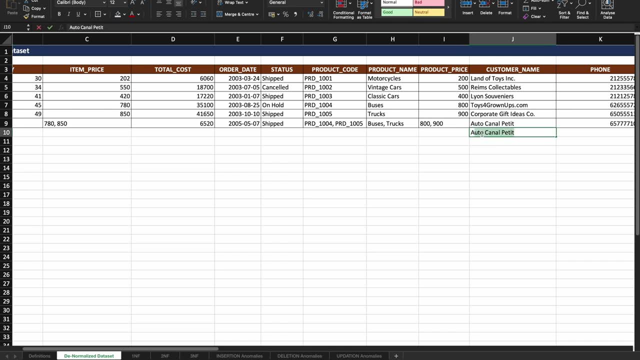 say that a is functionally dependent on c. okay, something like that. Now let me explain that in simple words. so, for example, let me go back to my denormalized data set that I had initially okay, and here let's say that I'm going to consider my customer name as a okay. so this is a okay, and I'm 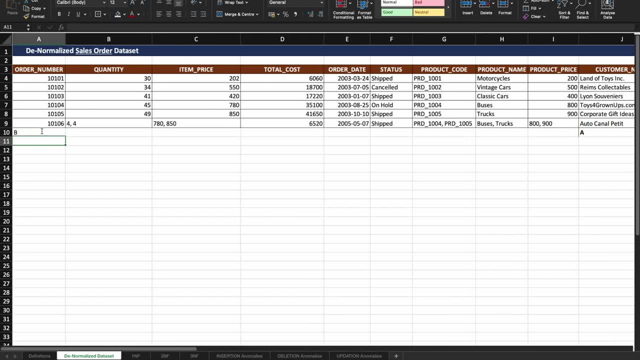 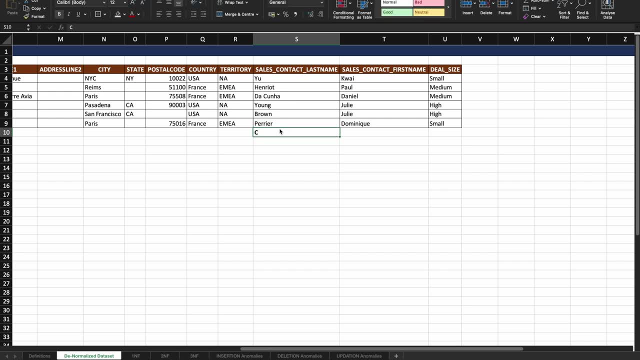 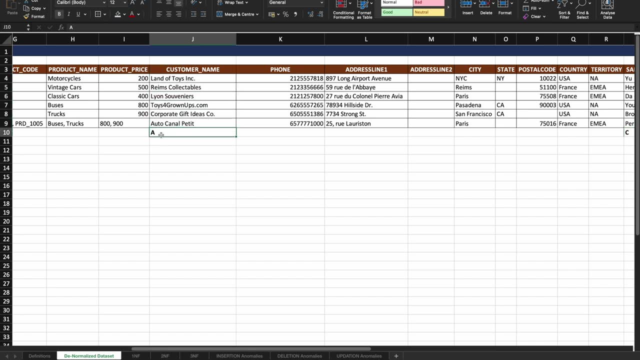 just going to mark it like a and let's say my order number is b- okay, and my sales contact name- this particular column- is c, okay, just for example. okay. Now, if I look at this data set, my customer name, that is my column a for this particular example. 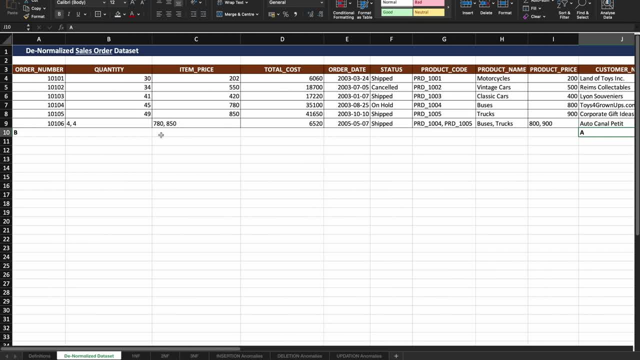 if I am aware of the customer name, then I can know what is the order that customer purchased right. So I can say that a is functionally dependent on b right. So basically, if I know a, I can know what order did that customer purchase right. Similarly, if I know b. so 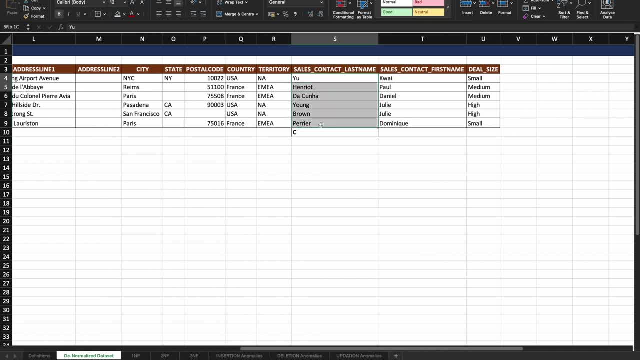 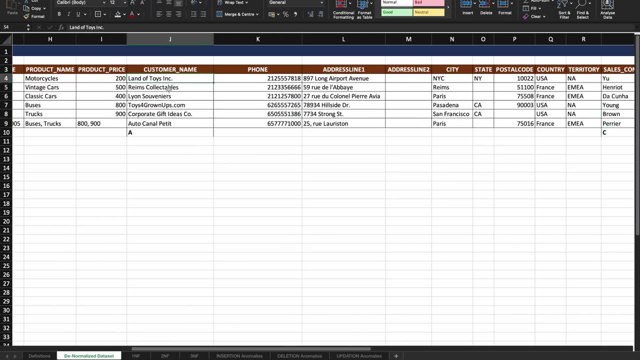 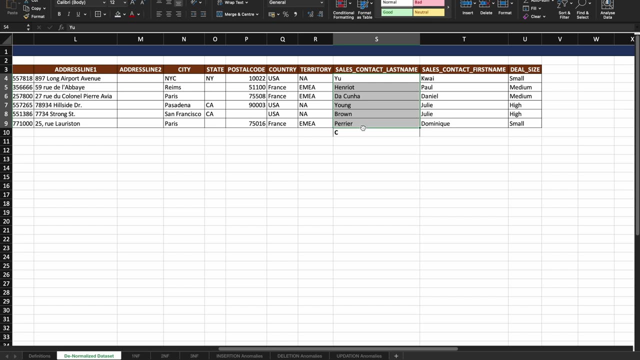 the order number, I can identify who was the sales person who was responsible for that order, right? So, since I know that? so in other words, I can say that if I know my customer, if I know a customer name, I can identify who was a sales person who was responsible for that order. okay, So this is. 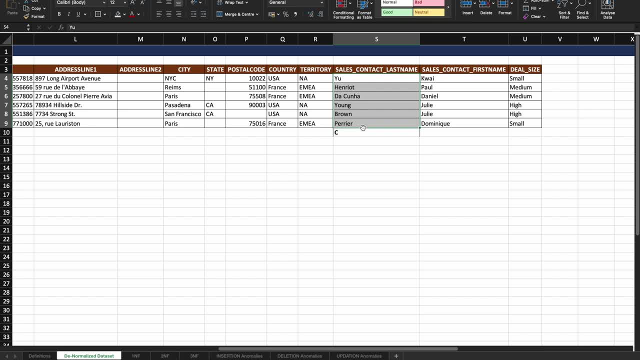 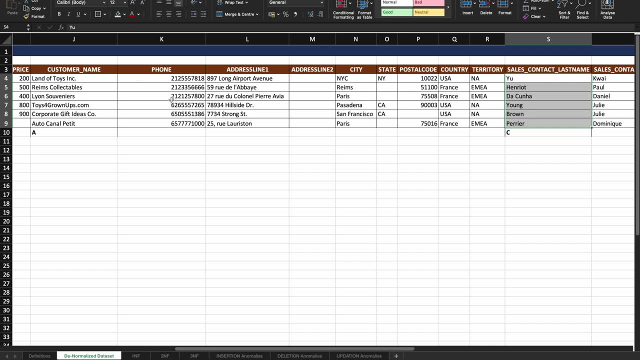 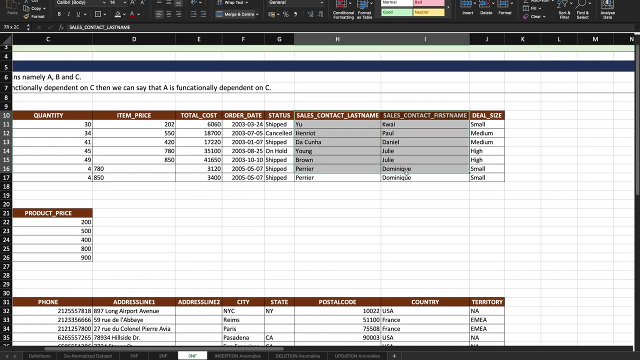 kind of like a transitive dependency that is present in this database. okay, So as as part of the second normal form, we have already split the customer information into a separate table. right, But if you look at the data set in the orders table, we can see that the sales person's information is. 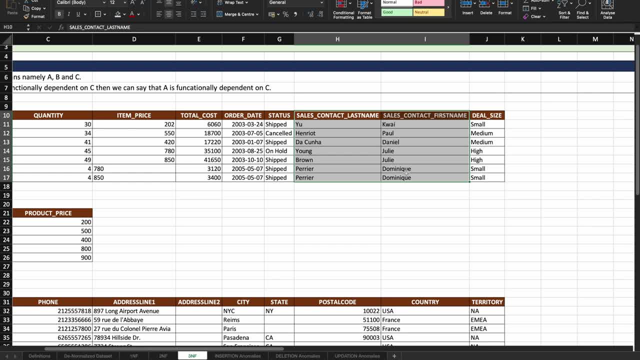 still stored in the orders table, which we basically need to remove and put it into a separate table, because this is causing the transitive dependency right. so what i'm going to do is i'm going to remove these two columns- that is, the first name and last name of the sales person- and i'm going 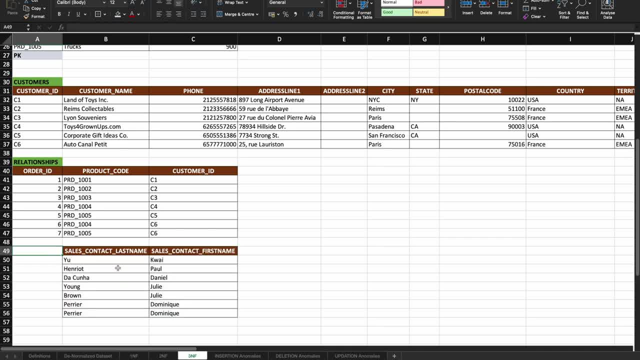 to create a separate table here. okay, and these sales persons are basically employees, so i'm just going to call, i'm going to create a primary key for this, for this particular data, which is going to be my employee id. now, before i create my primary key, i can see that there are some duplicate data. 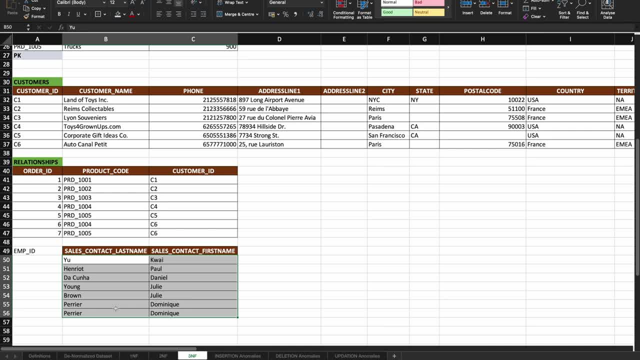 right, because two sales person might have might have been responsible for multiple orders, right? so i'm just going to remove the duplicate data because, since it's an employee table, i don't need to store the same employee information multiple times. so i'll remove the duplicate data and now. 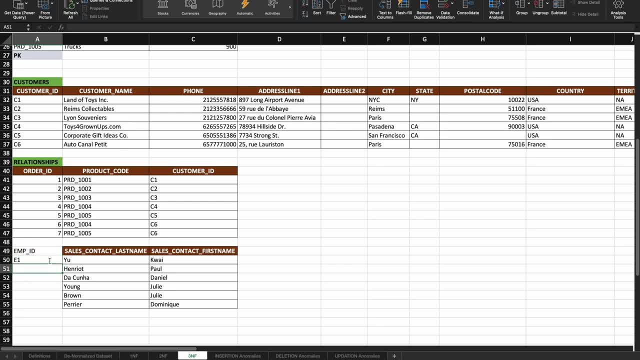 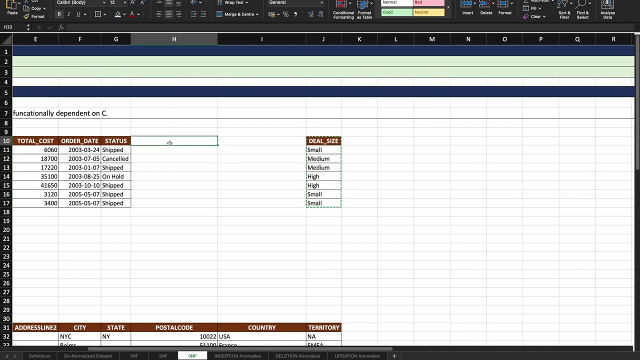 i'll add the primary key and i'm just going to say e1 until, uh, the last, and i'll just copy this formatting and i'll just put it here. okay, so this becomes my employee table. that is fine, and i'll just move my deal size column to the left so that it is. 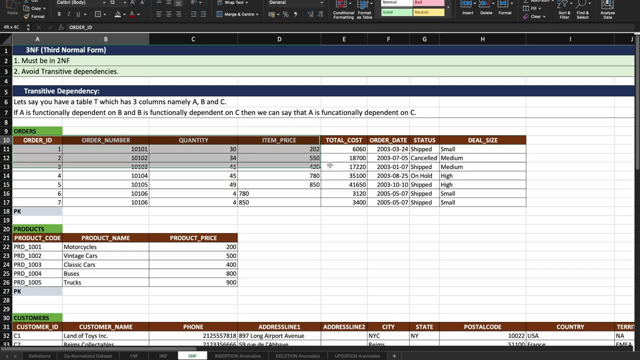 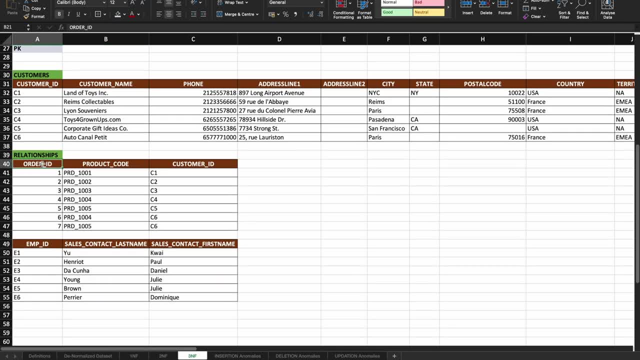 clearly visible in my orders table. okay, so now i think my orders table is perfectly fine. it has only order information. my products table is fine, customer table is fine, the relation table is fine and i have created employee table, but there is no relationship between the employee table and the 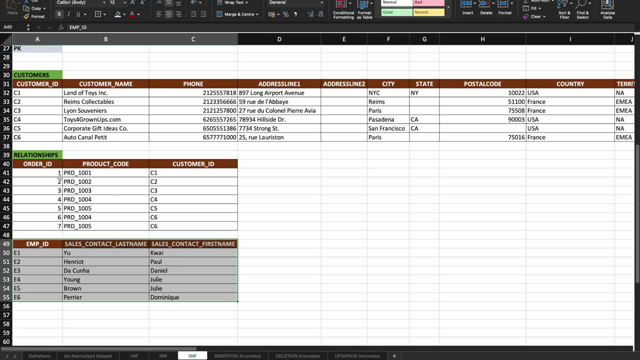 relation and the relationship table. so i'm just going to remove the duplicate data and i'm going to create my relationship table. now, how do i create this link again? what i'm going to do is i'm just going to copy this employee id and put it into the relationship table, and i know the last two orders. 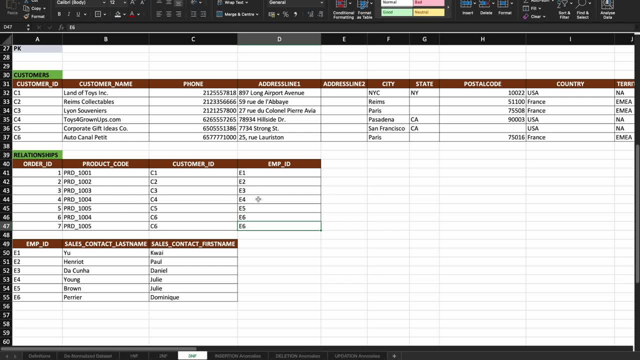 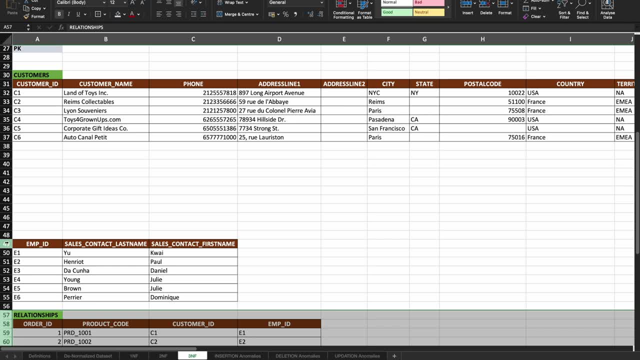 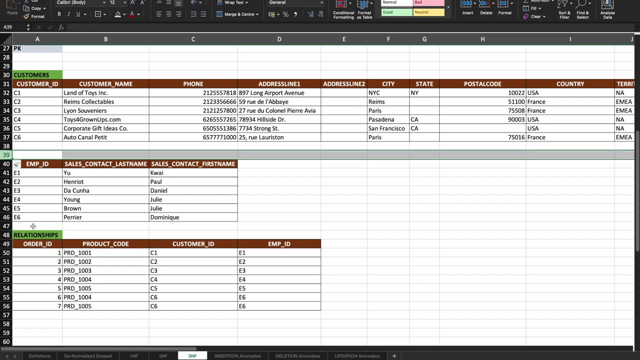 were done by the same employee. so i'll just make that update here, okay. so now i can say that, okay. so just to make it clear, i'll just move this to the down, okay, and i'll move this to the top here, and this is my employee table. 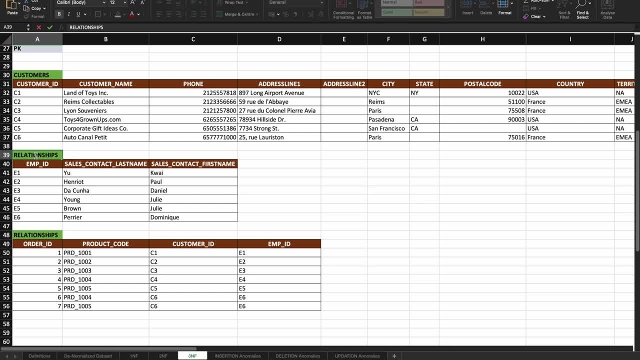 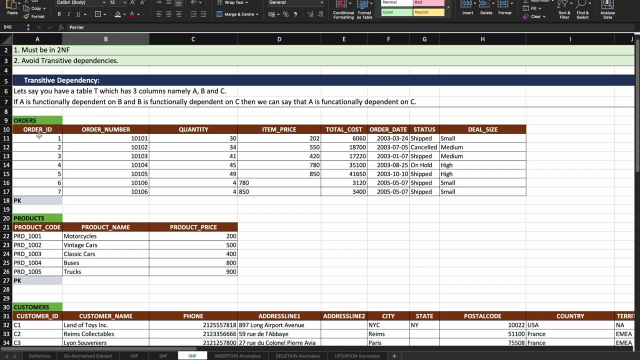 right, so i'm just going to put this relationship in that. okay, i'm meu. i'm just going to hide it here. okay, now i need to confirm everything so i can rename it, just to see the last two orders in a row. ok, it here and this is my employees table. okay, so now you can see that I have my orders table. 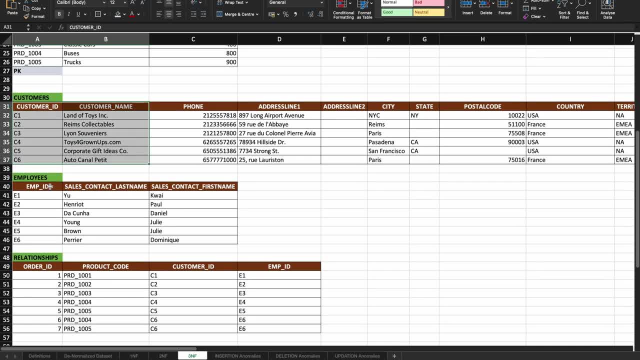 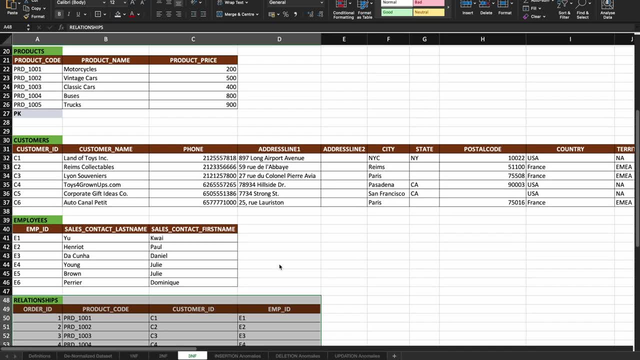 separated. I have my products table, I have my customers table, I have my employees table and, finally, I have a relationship table, basically, which provides a link between all of these tables. so this we can say, that now my entire data set is in third normal form which, as I said, is the 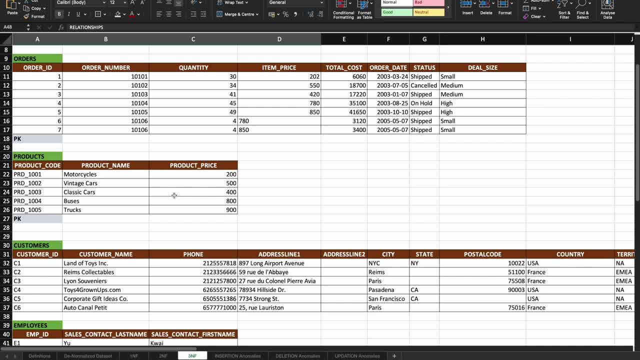 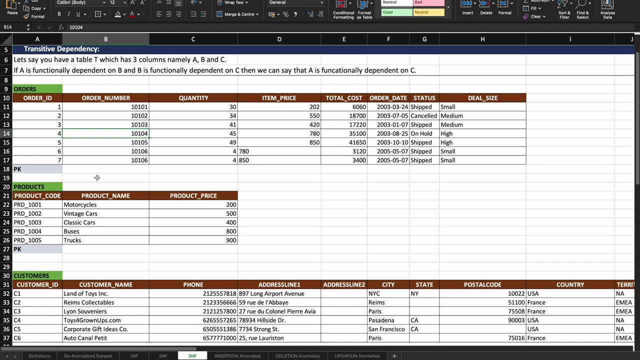 golden standard of normalization. this much or level of normalization is actually pretty good enough for almost any of the database that exists today, so I hope this is clear now. I think one thing that I forgot to mention about the foreign key is that maybe I did not explicitly mention that. 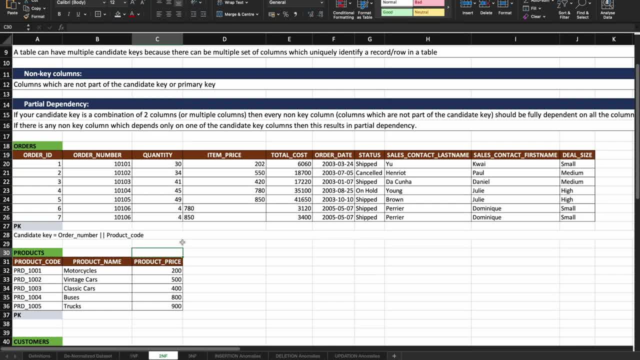 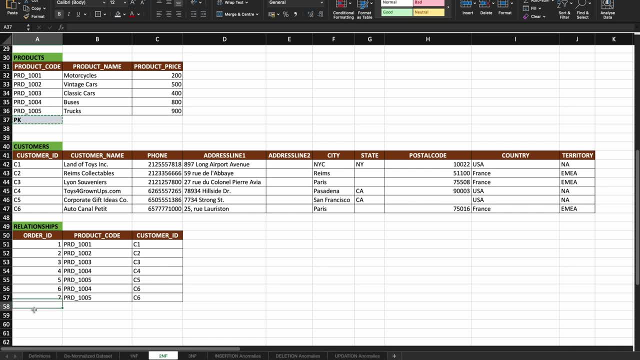 how did you create the foreign keys in the second normal form? because we created the primary keys based on the columns that I mentioned here. right, this was my pk column for my relationship table. orders id is the pk column for my customers table. the customer id is my pk column. 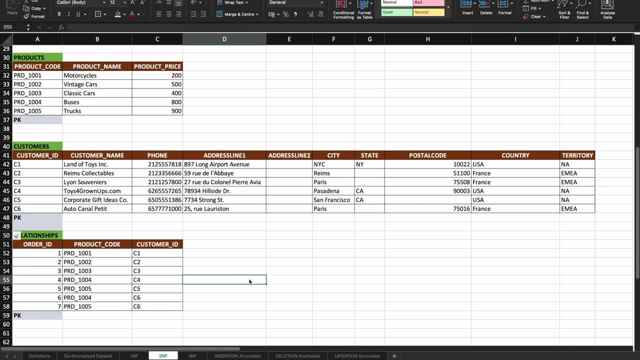 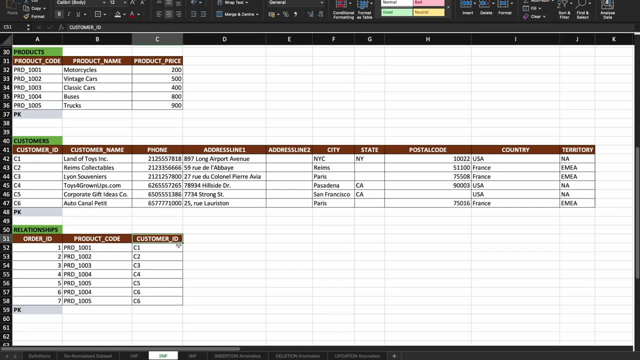 but where exactly is the foreign key right? and that is what i did not, i think, explain, so let me talk about that now. so, basically, when i say foreign key, it basically creates a master and child relationship. in in this particular case, my orders table is my master table, my products table is also. 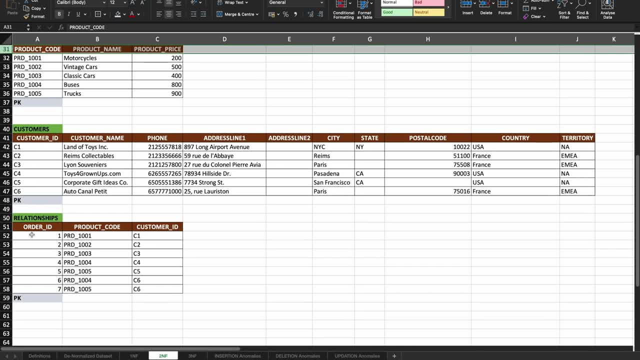 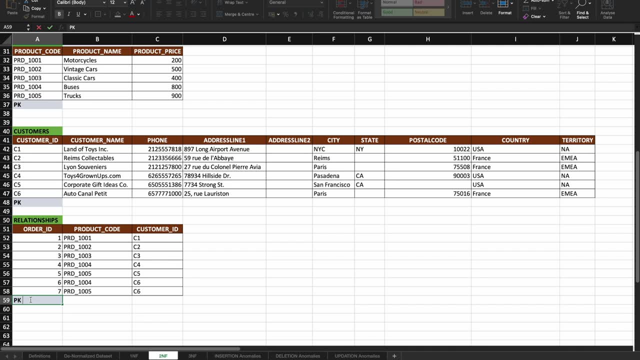 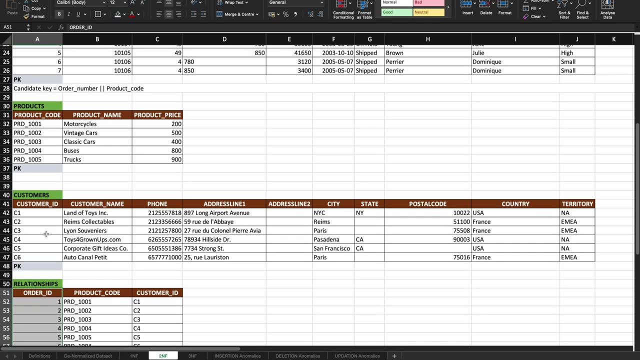 master table. customers table is also the master table, but this relationships table becomes my child table, right? so what i do? i create a foreign key here. so this will be my pk and my fk. so i create a foreign key for this particular column, which is going to reference the order id from the. 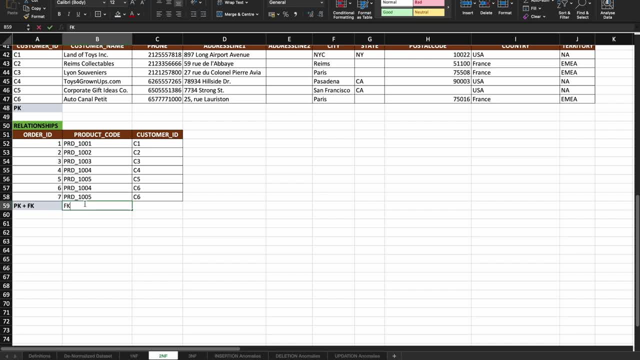 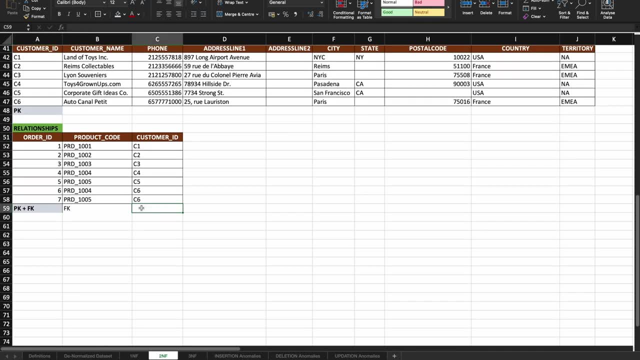 orders table. same way, i'll create another foreign key here, okay, which for product code column, which is going to refer to the product code from the products table. and i'll create another foreign key in my customer id column, which is going to refer to the customer id from the customers table. 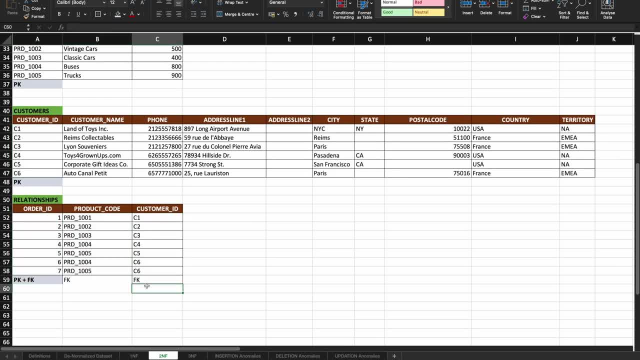 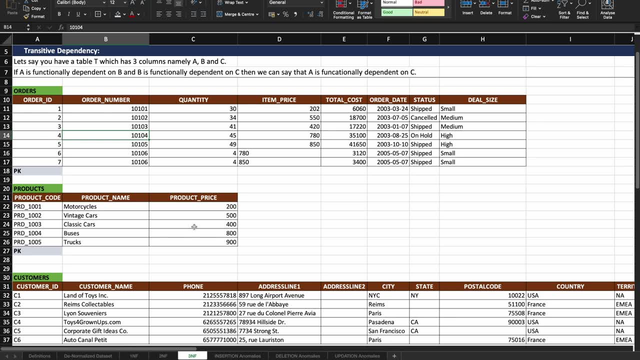 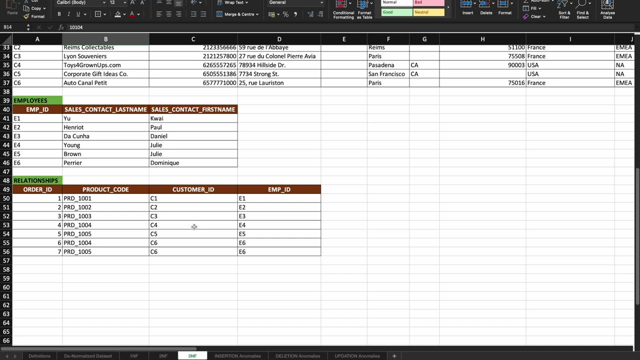 so my foreign keys are created in my relationships table. okay, i hope this is clear now. okay, now, this is the end of the section. you two: i hope you have completely understood the three levels of normalization and how we have normalized our denormalized data set into this level of normalization. okay, now let's move on to. 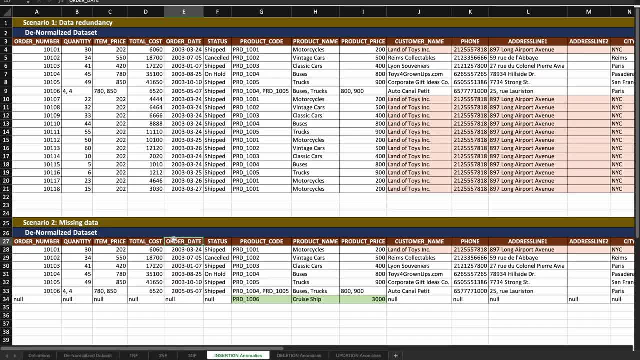 the last section where we'll be talking about the different anomalies. first of all, let's start with insertion anomaly. now, what exactly we mean by insertion anomaly is basically: anomaly means problem. we can say insertion problems that can exist in a denormalized data set. okay, so our 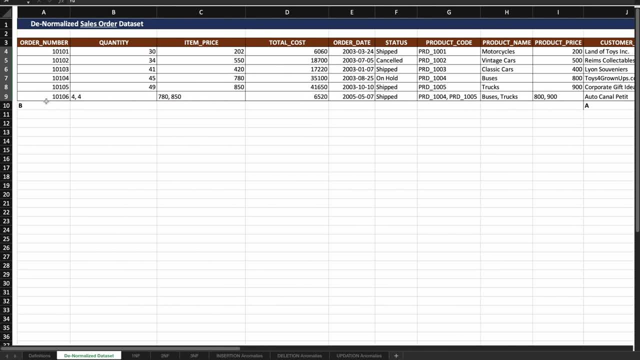 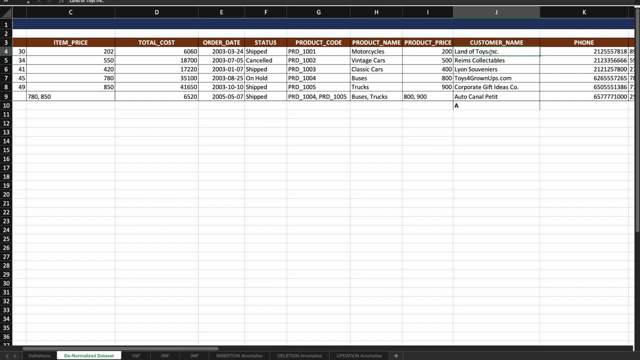 initial denormalized data set looked something like this: right now, let's say, one of the customers here is this one that is land of toys. okay, now, over a span of couple of months or some time, he or the, the company, would be purchasing multiple different orders. okay, and every time they purchase an order the order number would be different. the product: 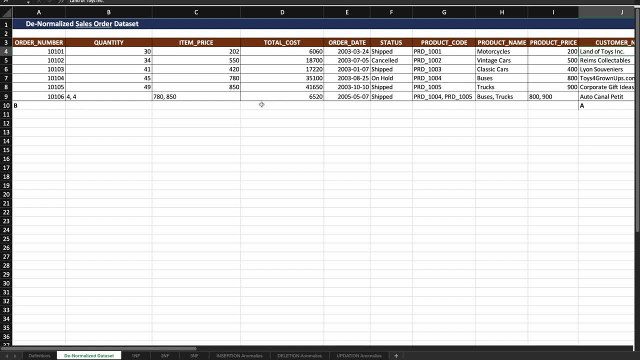 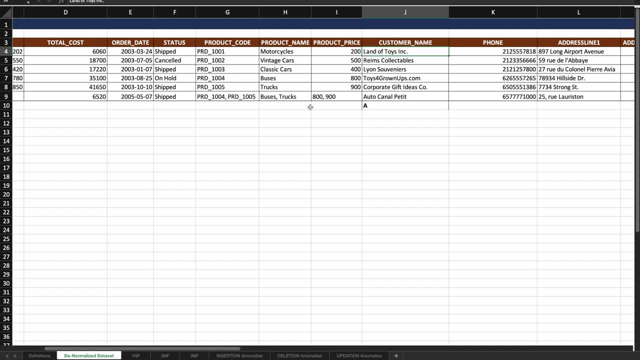 might be different, the price and everything else. date, everything would be different, but it's the same customer right so for every order. even if he purchases 10 orders or 100 orders or whatever the number of orders, their information would be different. right so for every order, even if he. 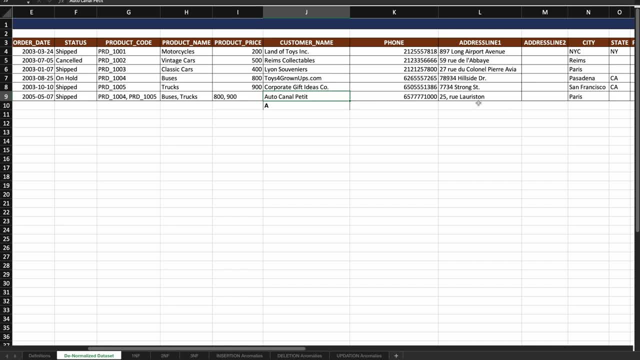 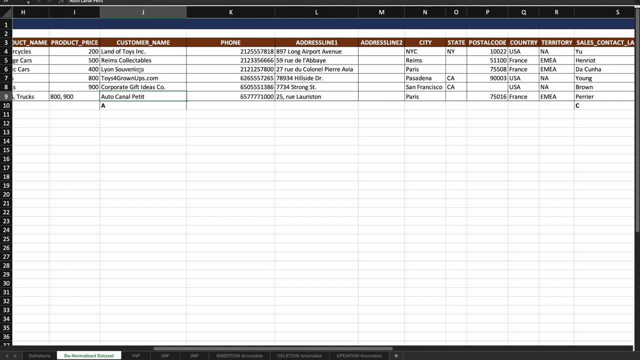 the customer information is basically the same, So the same information would have to be inserted into this table. Why? Because there is just one table right. This is a table which has information about a customer, about the order, about the product, everything right And the. 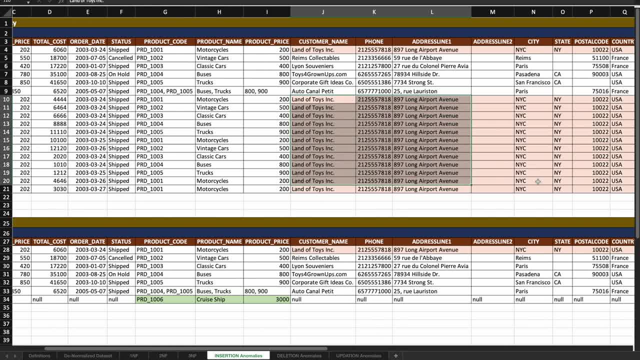 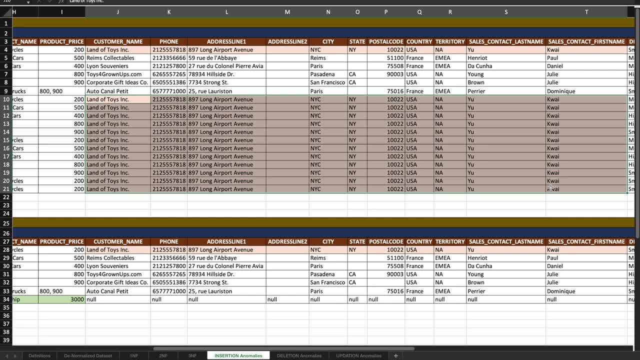 data would look something like this. So the same customer, his information, is basically getting repeated multiple times. Why? Because there is no separate table or place where the customer information would have to be stored right, So everything has to be in this denormalized table. 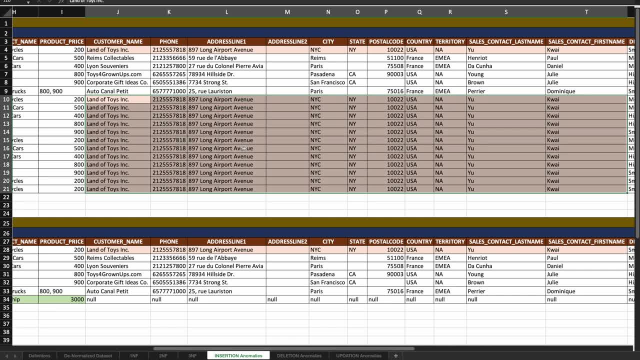 So some of this information would basically get repeated, which basically results in data redundancy, And this is one of the insertion problems or insertion anomalies that can exist in a denormalized data set. okay, Now let us say if we have to do this same activity in: 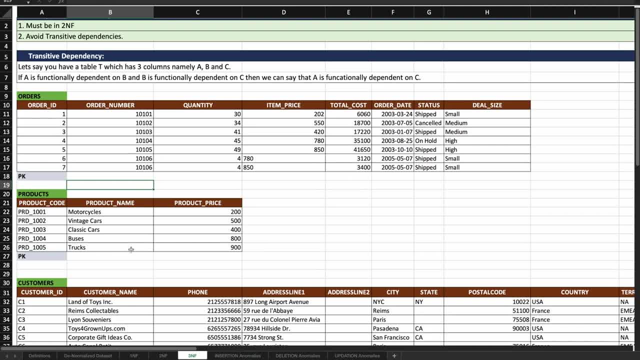 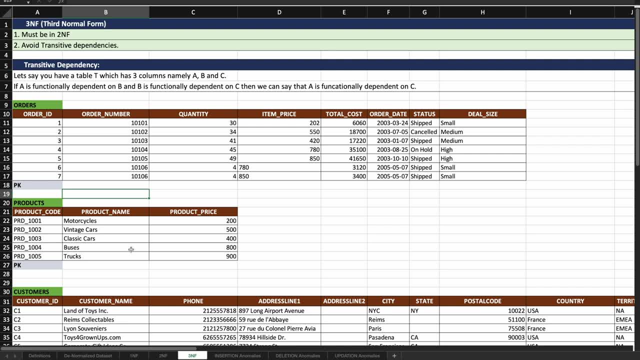 a normalized data set, for example, the third normal form that we discussed in the earlier section. we came up with these set of tables. right Now let us say this is the database that we have, the normalized database as per the third normal form, And this: 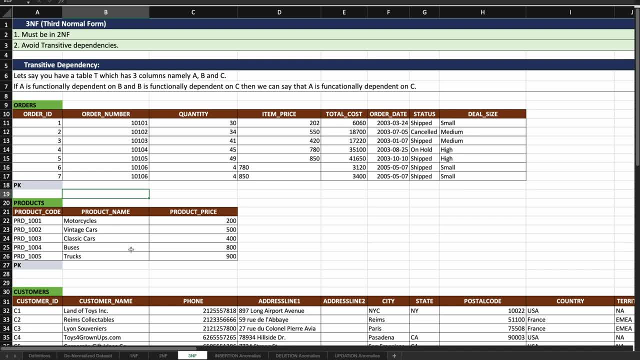 is where that particular customer is going to purchase multiple different orders. So whenever that customer- that is, let us say the customer- is land of choice, he or they want to purchase multiple orders, all their order information just gets inserted into this orders table. 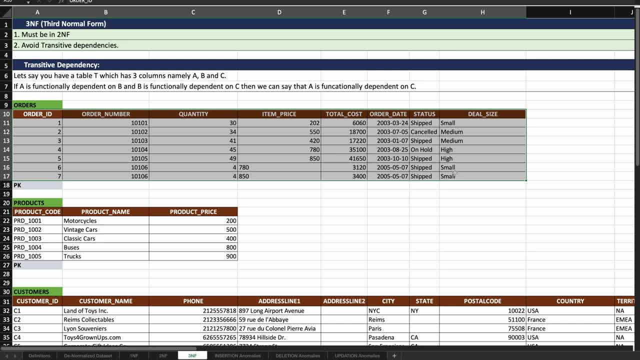 right. Whether it is a 10 orders, 100 orders or whatever number of orders, everything only has to get inserted into this table. There will be no changes into a product, because these are all the existing products. They are not going to be inserted into this table. So this is the. 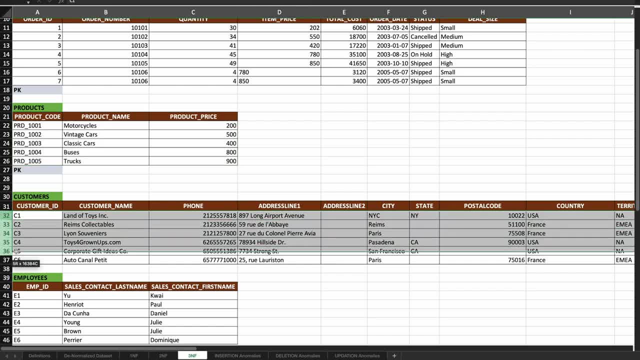 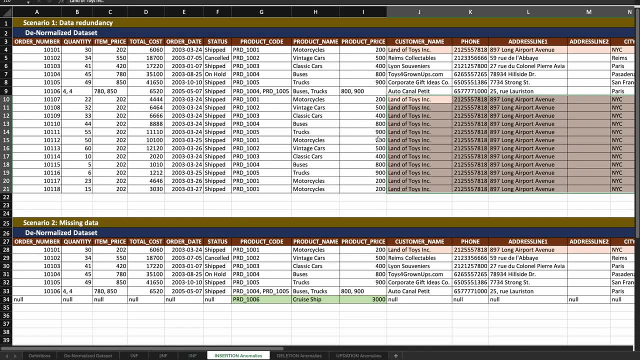 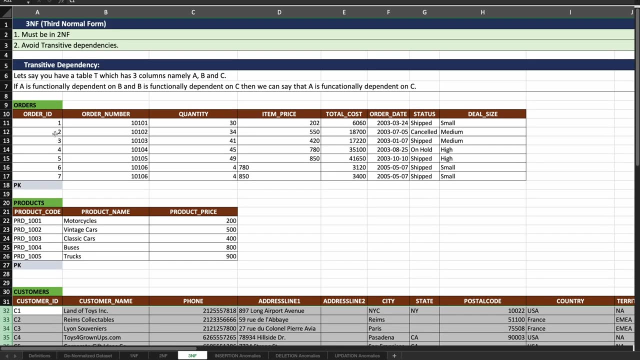 data that we are purchasing And there is no info, no changes to the customer information, because the customer table already has their information right. So the data redundancy that was caused in this denormalized data set is basically completely eliminated because of the normalized level of database that we have here. okay, I hope you understand this. 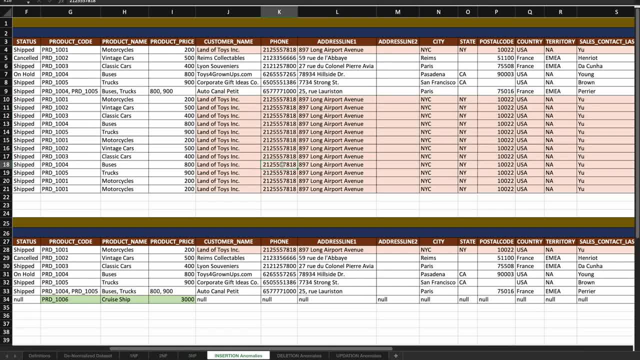 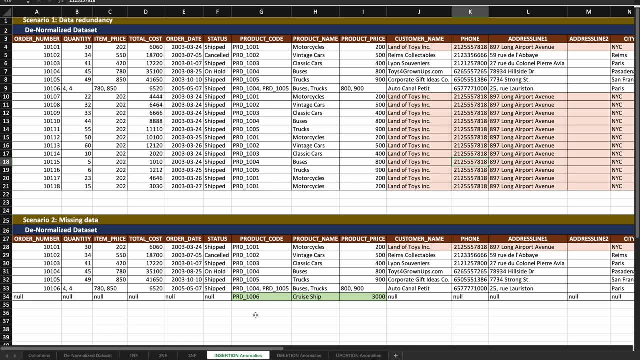 particular concept of insertion anomaly. okay, So this is just one scenario. Now a second scenario could be that let us say there is a customer who has purchased multiple orders change in the product, So let us say a new product has been introduced by the company. 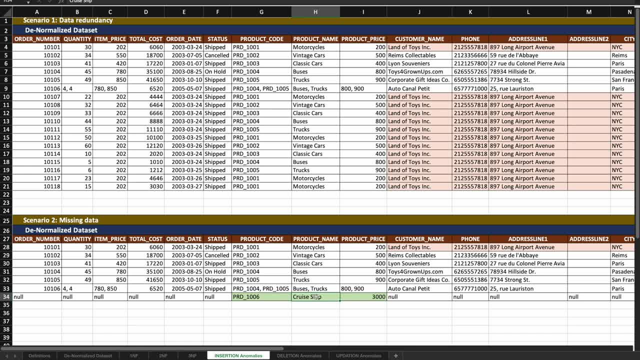 and maybe it is a cruise ship. Now they want to insert this cruise ship information into the database. and, let us say, you only have denormalized data set. Now, in a denormalized data set, when you want to insert the information about a specific list of values, that is, let us say, in this case, 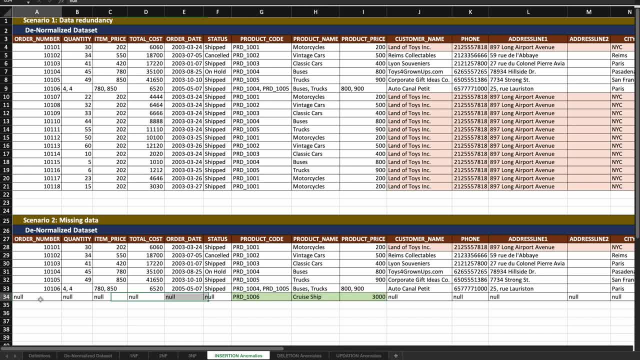 product. you have the product information, but there is no orders for that, No one has yet purchased this product. So no one, no customer, has purchased this product. It is just a new product introduced by your company. Now, in order to add this into your database, into your 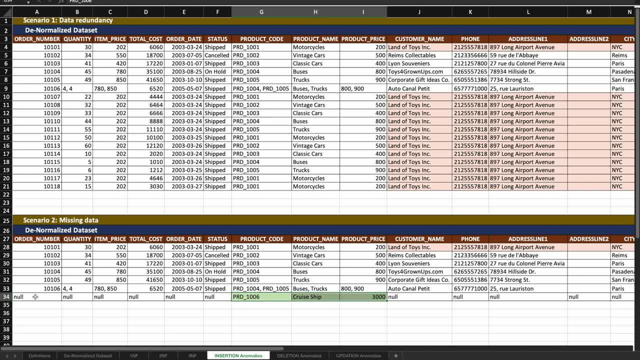 denormalized database. you have information about the product, but there is no information about the order, There is no information about the customer, So all of this would have to be null, which is basically not right. So in order to just insert a product, there is no other place you could just. 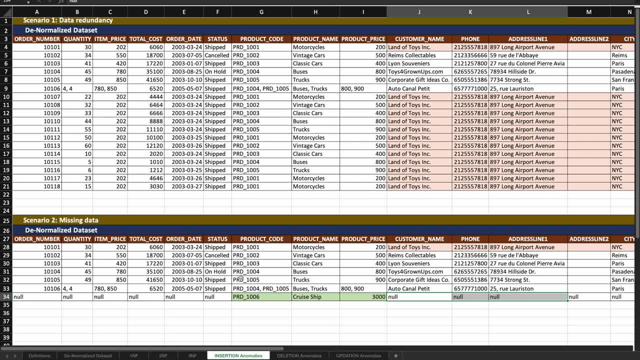 enter information about the product, You have to use the same denormalized table where lot of the other columns has no value, So it would basically be blank, which is again is causing missing data here. So this is also a form of insertion anomaly that can exist. Now let us say: 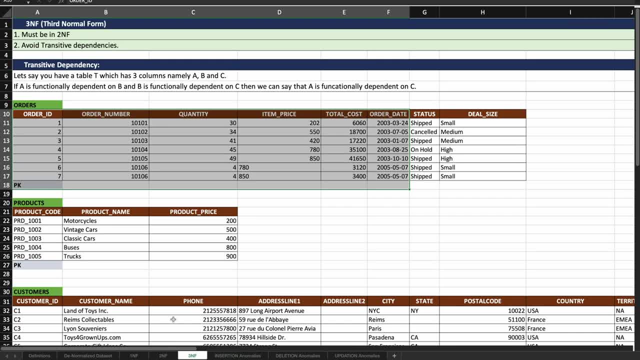 if we have to do the same activity in a normalized database. that is this third normal form data set that we have created Here. if I had to introduce a new product, I could simply add a new record into this products table. Just add a new record into this products table and everything is done. No, 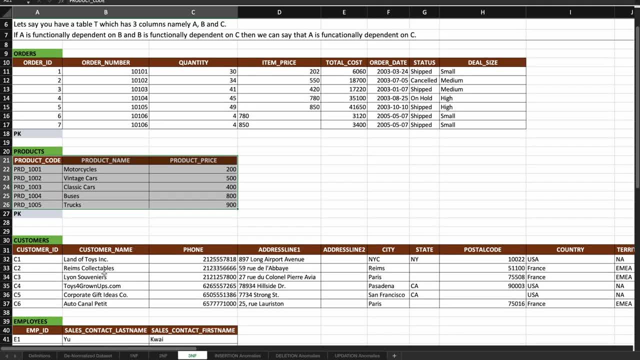 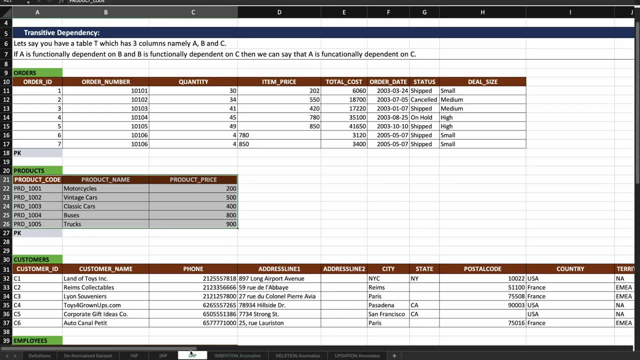 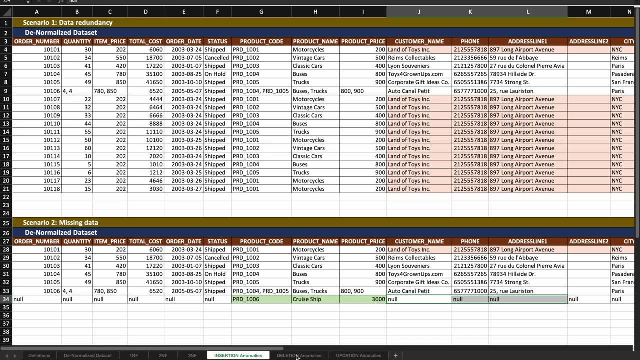 changes to the orders, No changes to the customers, No changes to the employees, etc. So this is how the second scenario in the insertion anomaly that can exist can be easily eliminated if you have a properly normalized database. So I hope the concept of insertion anomaly is clear. Now let us move on. 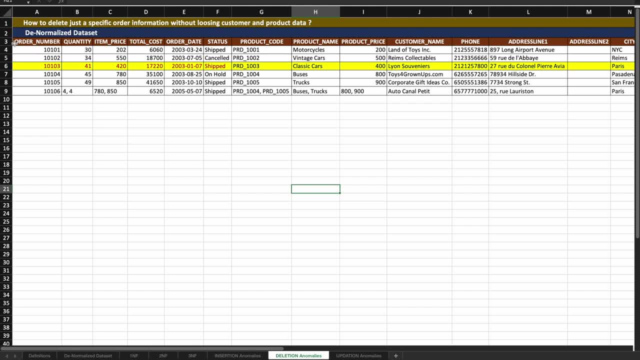 to deletion anomaly. Now let us say you have this denormalized database and let us say you have one of the requirement where, due to whatever reason, you have to remove one of the orders from your system. Maybe it was wrong, So you have to remove this particular order. that is 10103 order number. You have to remove it. Your. 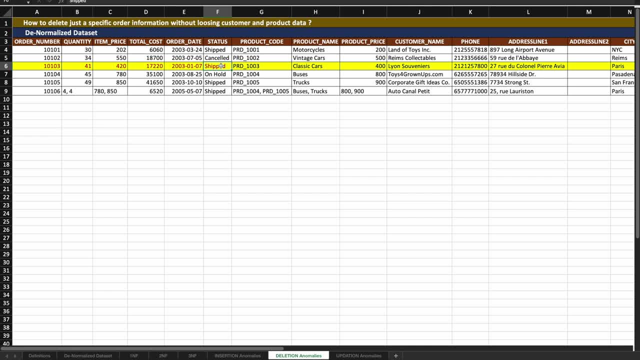 intention is only to remove the order from your database, But if you have to remove this order in the denormalized data set, you have to remove this entire record. When you remove this entire record, you are not only losing the information about the order, but you will also lose information. 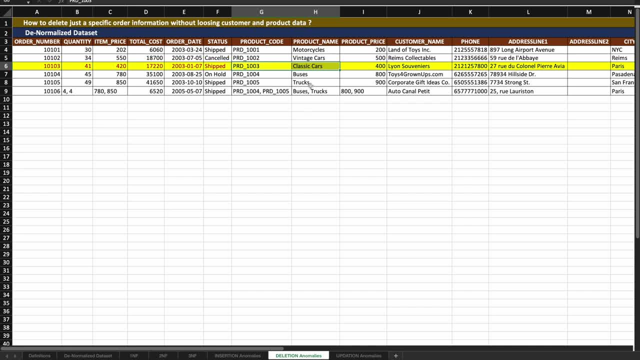 about this product. You can see that this product- classic cars- is only present in one of the records, one of the record in this table. So if you delete this record, you have to remove this entire record, This order record. you will lose this product information completely or permanently from your. 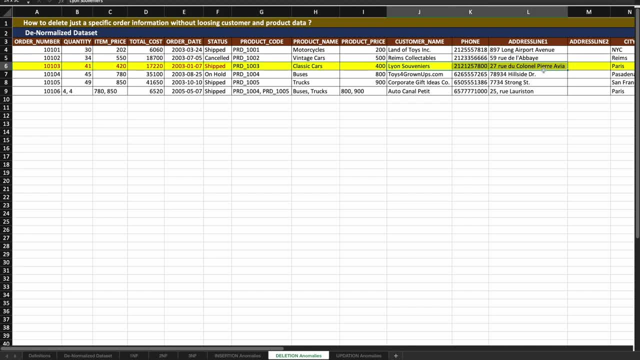 system and the same thing with the customer. This customer is only present in this record. If you delete this record, you are not only losing the order information, you are also losing the product information. you are also losing the customer information, which is actually not right. You 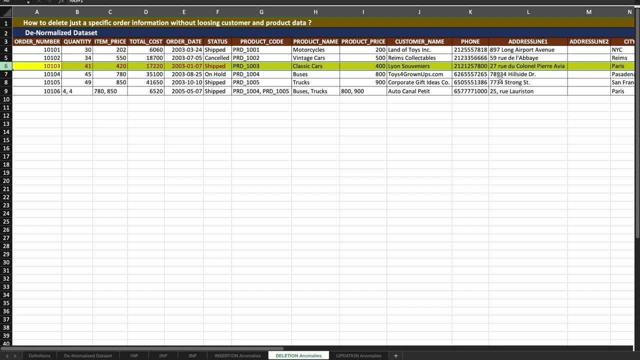 only if you want to remove something, you should know what you want to remove. Ideally, if you want to remove an order, that is fine, but you would definitely not want to lose information about your customer or about some product that you have. So this is a problem of deletion or deletion anomaly that can exist in a denormalized data set. 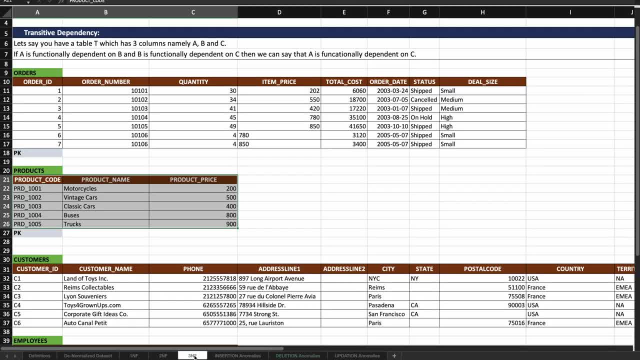 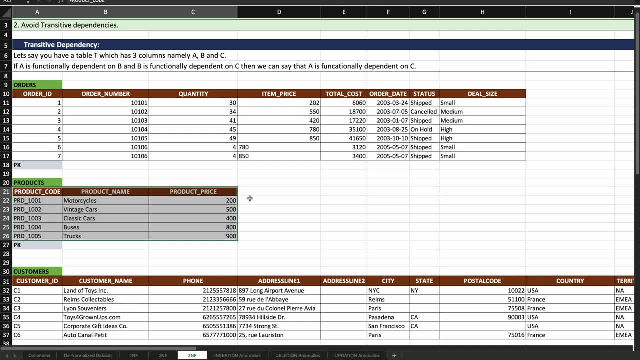 Now let's see how we could easily do this in a normalized database. Now again, I'm taking this third normal form data set that we have and let's say we have to remove one of the orders, And the order that we had to remove was this one. So here I could easily come to the orders table. 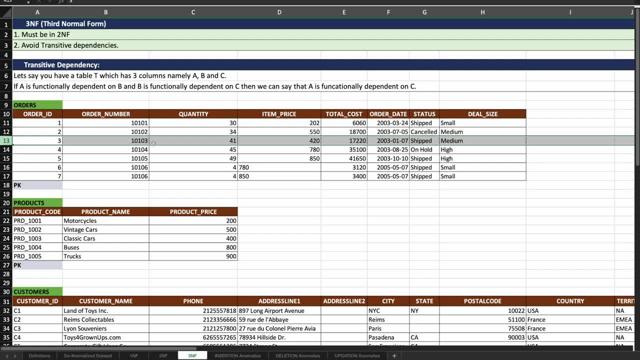 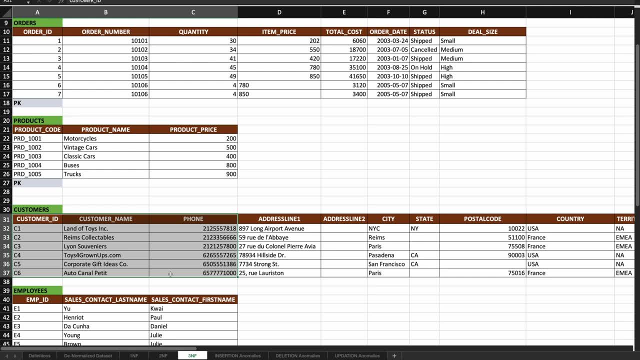 and I could delete this order And once I delete this, I have no changes. Basically, it does not impact my products table. It does not impact my customer's table. So these are the two things that table. so, basically, I am not losing any additional information, I am only losing the information that. 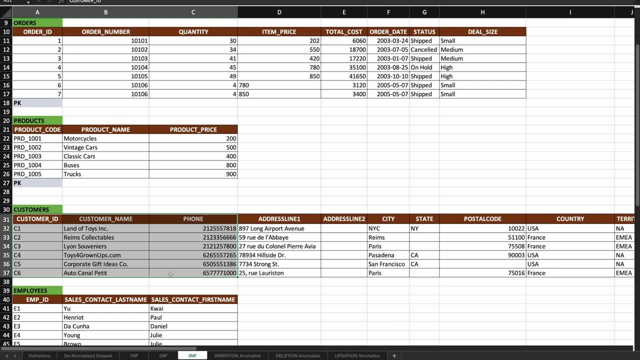 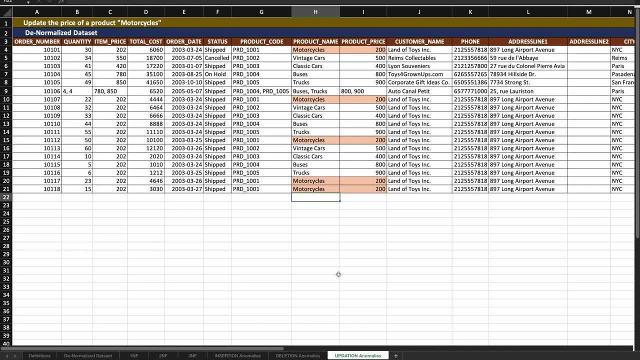 I actually want to lose right. so this is basically how your normalized data set is going to avoid deletion anomalies. okay, I hope this is clear. now let's talk about updation anomaly. okay, now again, it's a simple example. let's say you have this whole data set, okay, so there are this many different. 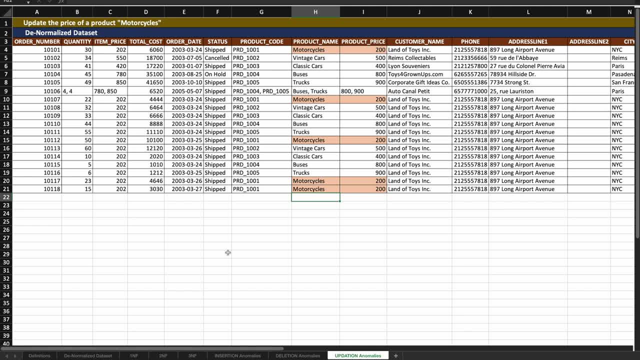 orders, and many of these customers have purchased motorcycles. okay, now, let's say there was a change in the price of your motorcycle. so someone said that the current price was 200. you need to change it to 250. okay now, if you have to make this change, ideally you would want this update to happen only. 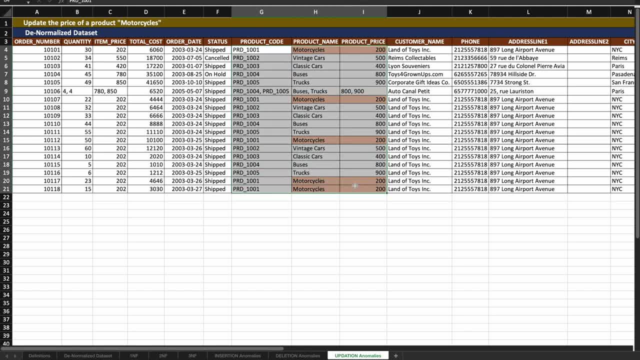 in one place. okay, now here you could see, probably I have some 20 records in real database. this might be 20 million records, okay, and this motorcycle might have been purchased with, let's say, 100,000 people. okay, if you have to update the price, you will have to update all the 100,000 records where. 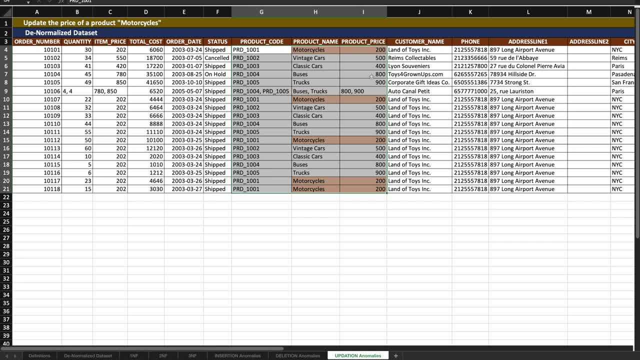 this motorcycle product was purchased right and that is not going to change in the price of your motorcycle. so someone said that the current price of 200 is not efficient. unnecessarily you have to update so many different records, whereas ideally there should have only been one particular place where you should have updated the price of your vehicle. 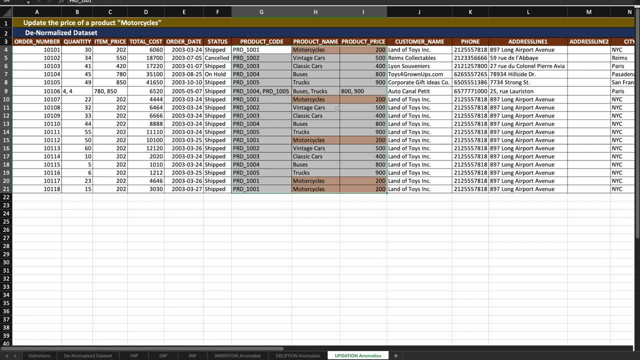 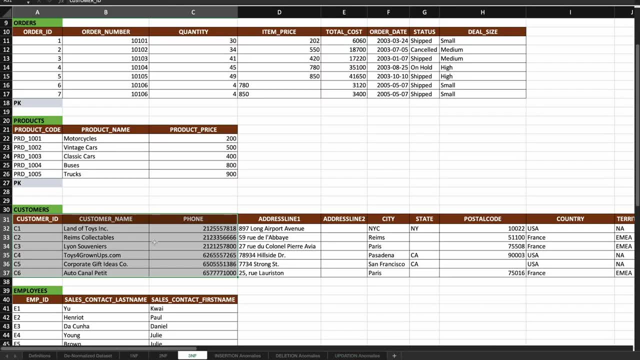 or your product, right? so this is a problem of updation. so updation anomaly that exists in a denormalized data set, but let's say if we have to do similar update in a normalized data set. here you can see that I just have one table for products. if I have to change the price, 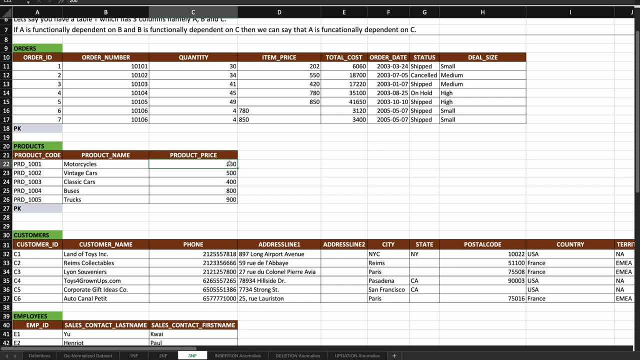 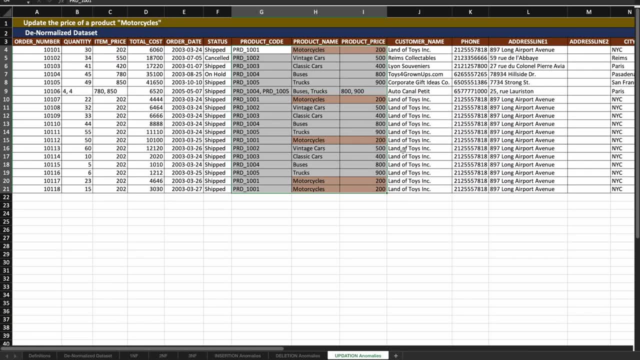 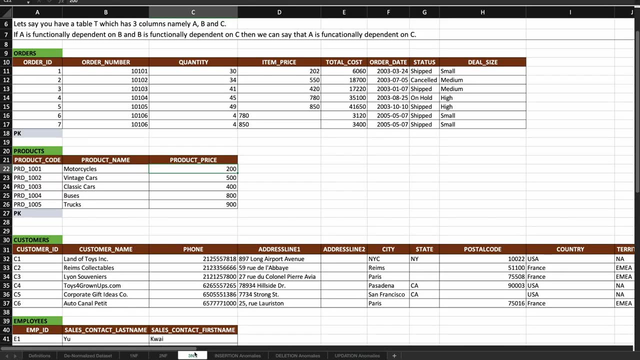 I just go into this one record and I update the price here. just one record will get impacted, right? so this is so much better than having to update the multiple records every order where the product was present, right? so this is basically how update anomaly can be avoided by using a normalized 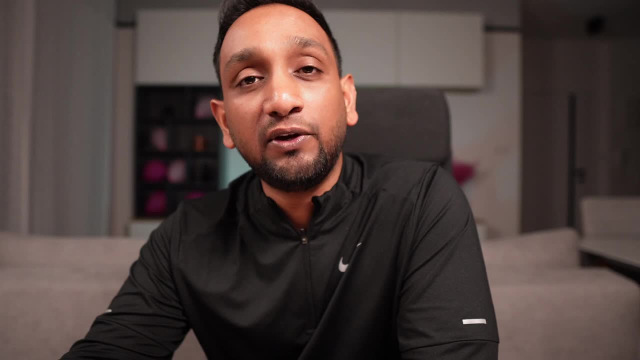 database okay, so I hope you learned something useful from this video, if you did definitely leave your feedback in the comments below. thank you so much for watching and see you soon in the next one. bye.